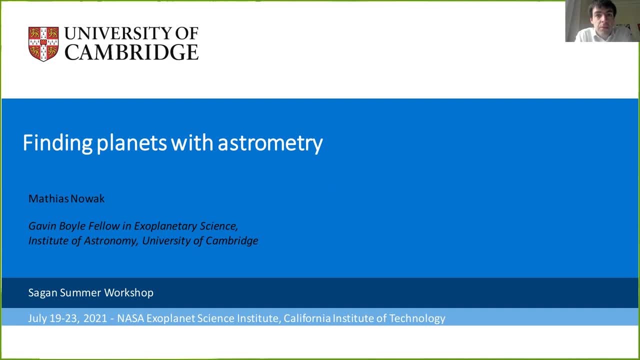 baseline interferometry And I am mainly working within the ExoGravity Large Program, which is a large program on the Very Large Telescope Interferometer dedicated to observations of exoplanets, And so with this program we've observed a number of planets so far and we've obtained a number of high precision astrometric measurements on 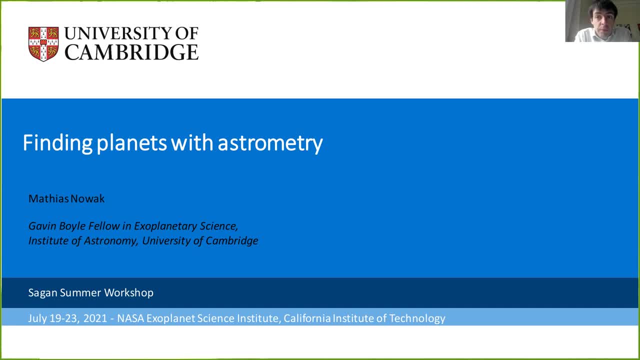 exoplanets, which I am going to talk about later on in this talk, But this is, of course, directly related to the topic I'm going to discuss today, which is finding planets with astrometry. And before I jump straight into the subject, I think it's good to start by saying that I am a professor at the Institute of Astronomy at the University of Cambridge, in the University of Cambridge, And I am also a professor at the University of Cambridge, at the University of Cambridge, And I will just say a few words. 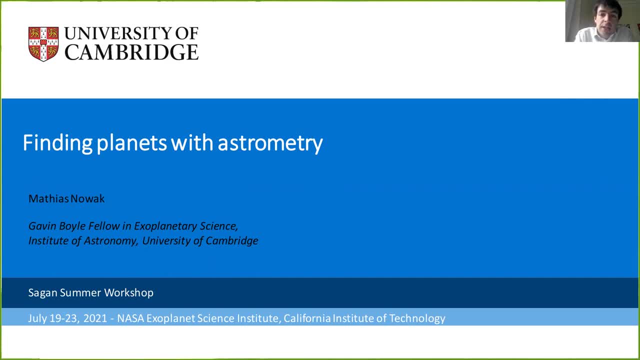 about the method into set the scene. So this idea of finding planets by looking at the reflex motion of the star isn't something new. It's actually quite an old idea But, to say the least, the beginnings of this method weren't really great. A number of planets. 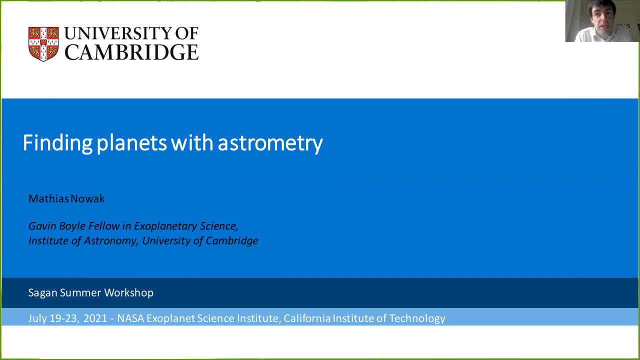 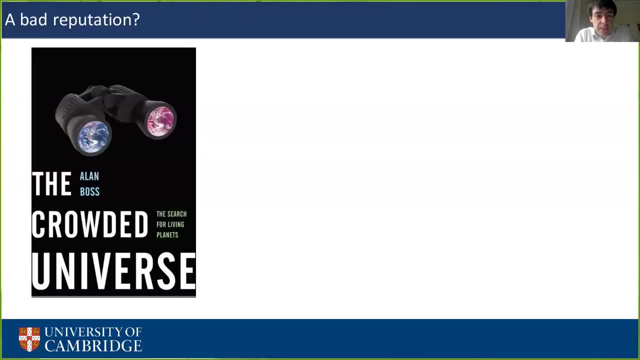 have been claimed in the past with this method, which turned out to be false detections, and so i recently came across a a book. it's called the crowded universe. it's written by alan boss, it was published, i think, in 2009 and it's it's not just about astrometry, it's really. 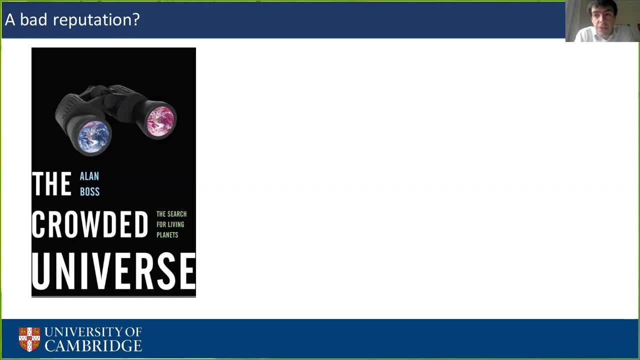 about the, say, the, the history of uh, exoplanet observations, the, the beginnings of the of the field, and. but there is a part in the book where, uh, the author talks about astrometry. um, and it's interesting because alan boss is an astrophysicist, so the book doesn't talk only. 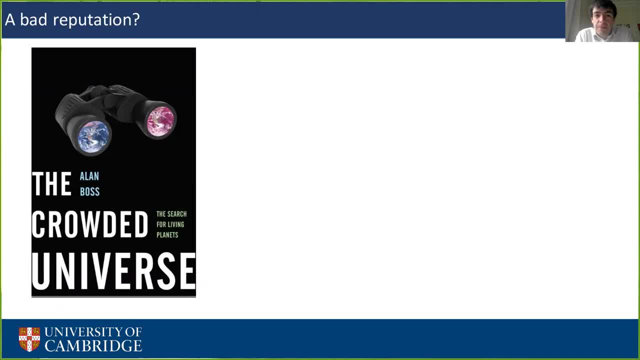 about the methods and the results, but it also gives sort of an inside view. and when he talks about astrometry so he explains that a number of detections have been may claimed in the in the past which turned out to be false detections, and then he writes, uh about astrometry. he 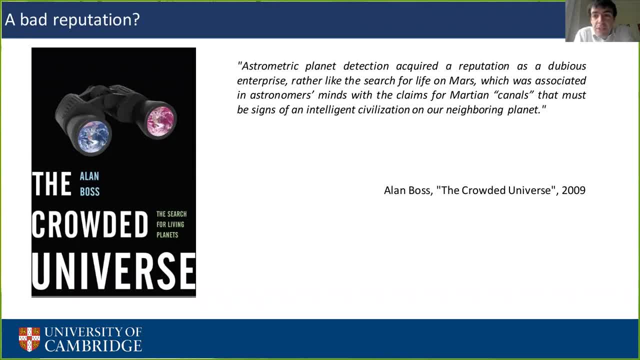 writes that astrometric planet detection acquired a reputation as a dubious enterprise, rather like the search for life on mars, which was associated in astronomers minds with the claims for machine canals that must be sign of an intelligent civilization on our neighboring planet. then he goes on and he says proper astronomers did not stoop to looking for planets or searching. 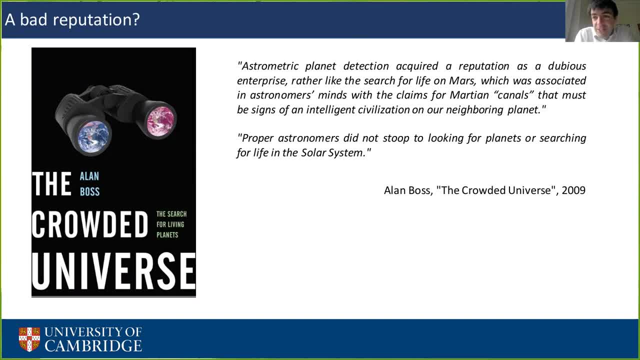 for life in the solar system. so that was written in 2009, which i think is interesting, and it raises one question, of course, is what is different now? i mean, we went from this state of mind, probably in the in the 2000s, to today where we have a dedicated talk on astrometric planet. 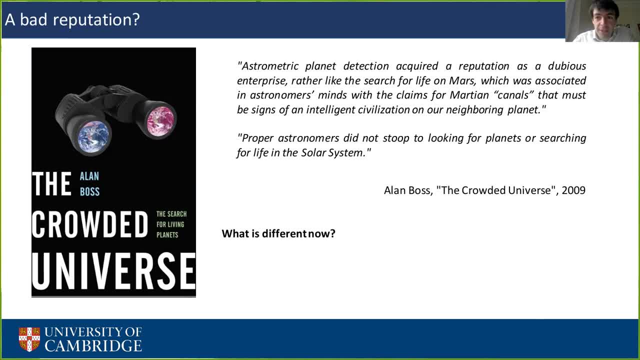 detection at the second summer workshop. so something, something must have happened for us, and i think there are two main reasons for for this change, which are related to two instrumental progress, basically. so the first one, of course, is the uh, the event of space-based observatories. astrometry is extremely difficult to do from the ground, of course, because of the 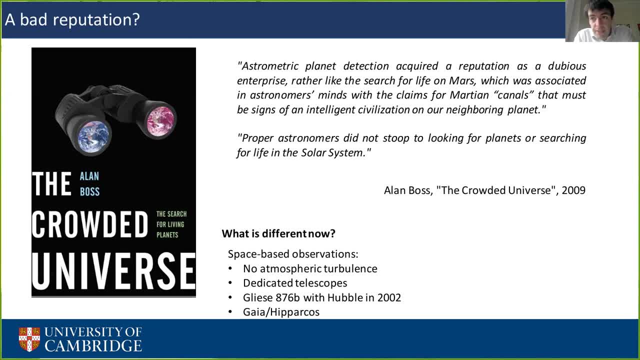 atmosphere. it's much easier to do this properly from space, and so, of course, the fact that we now have even dedicated space-based observatories to do this- i'm thinking of gharial- really changes, changes the the situation. and the second, uh, the second one is long baseline interferometry, um which we now have long baseline. 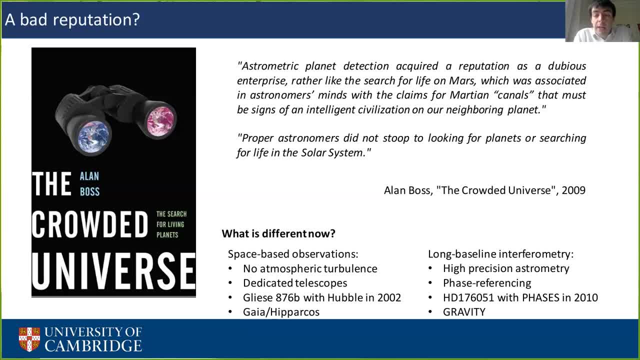 interferometers which are working very well, and from the ground, long baseline interferometry is one of the methods which can give the best results in astronomy. you can get really high precision measurements with this technique from the ground, and so there's two different methods to do high precision strometry are basically going to be the two paths of my talk today. 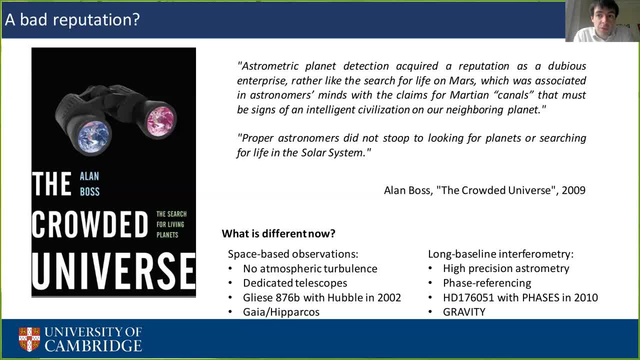 so i'm going to talk mainly about this combination of gaia and hipparchos data, which are two space-based observatories, and combining those data can lead to the detection of new planets. so that's something i'm going to discuss quite extensively, actually, and then, in the second part, i'm going to 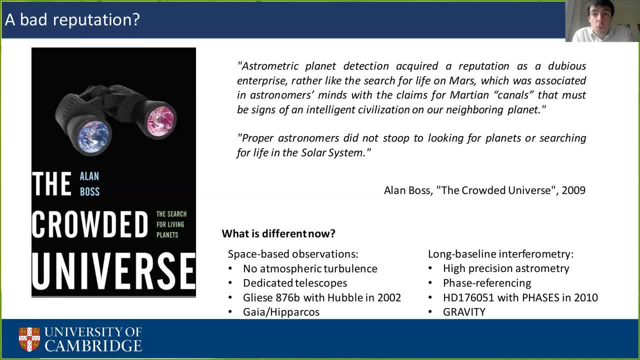 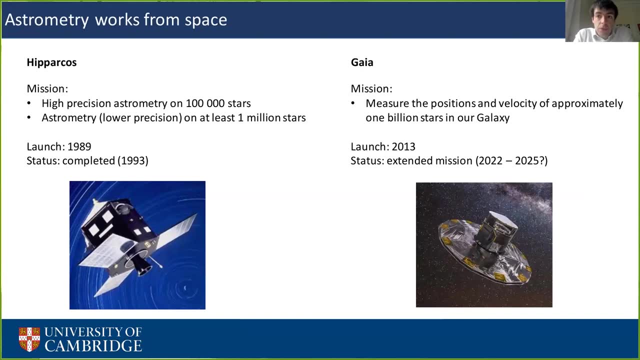 focus on uh gravity and what uh space-based observatories are going to be able to do um, and what long baseline astrometry can also bring to this topic of finding planets with astrometry. So, Gaia and Hipparchus. So Hipparchus is a satellite which was launched in 1989 and operated until 1993.. 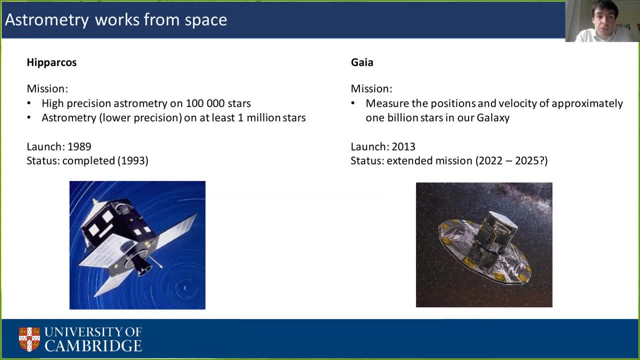 It's a European satellite and the mission was to get high precision astrometric measurements on the number of stars. I think the last catalogue has something like 2.5 million objects in it, But there are only 118,000 stars on which high precision astrometry is obtained. 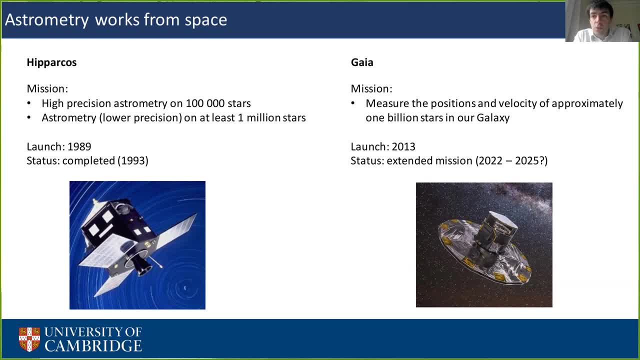 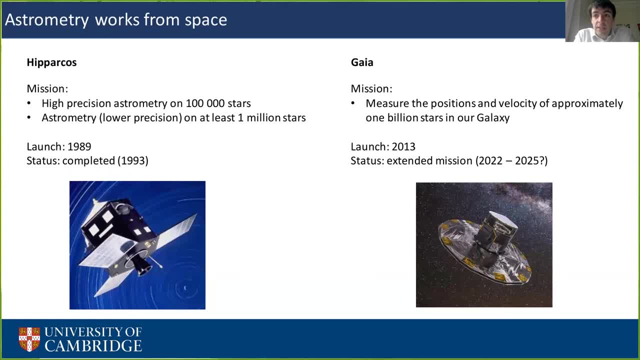 This is, of course, a much more recent satellite and the number of targets is huge and the precision obtained is excellent. So this is really, I think the combination of those two missions, is really the foundation of what I'm going to discuss today. I think it's fair to say that if it wasn't for Gaia, we wouldn't be talking about this. 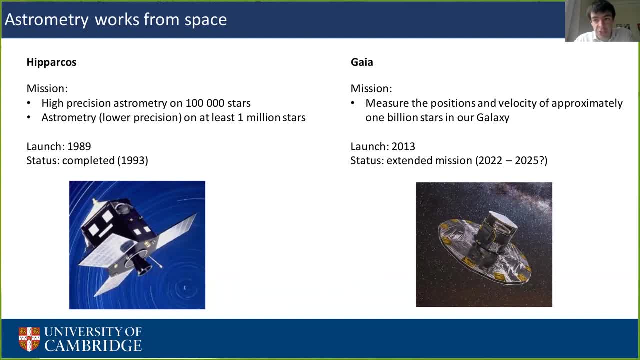 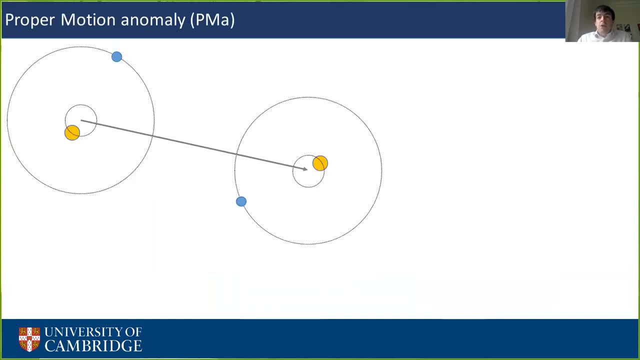 properly. It really changes. It changed. It changed many things in the field of astronomy. So how do we detect planets? using Hipparchus and Gaia and astrometric measurements, So one method which is probably the most used is. So the idea of astrometry is looking at the reflex motion of the stars. 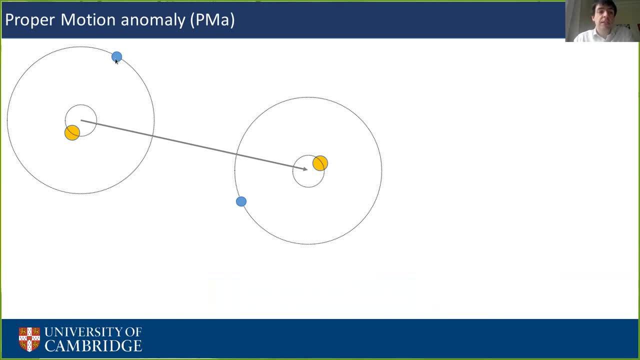 So if you have a star in yellow here and a planet in blue orbiting around it, the planet is now orbiting around the star star. it's orbiting around the center of mass of the system, which means that the star itself is also orbiting around the center of mass. so there is- uh whatever? a reflex motion of the star caused. 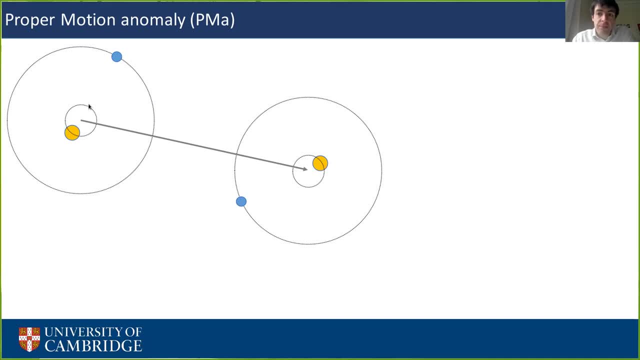 by the presence of the planet. now, of course, the whole system can have um its proper motion. so the whole system can have a motion on the star, and so the motion of the star is going to be a combination of the two, combination of the reflex motion caused by the planet and the long-term motion of the 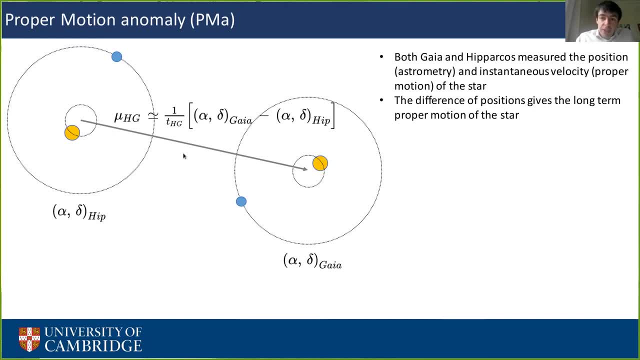 system. so, using hipparchus and gaia data, it is possible to measure this motion, and one thing you can do is um. so hipparchus obtains geometric measurements on stars in, i think, the reference epoch is 1991.. whereas gaia obtained measurements at the reference epoch, which is 2016, at least for for dr2. 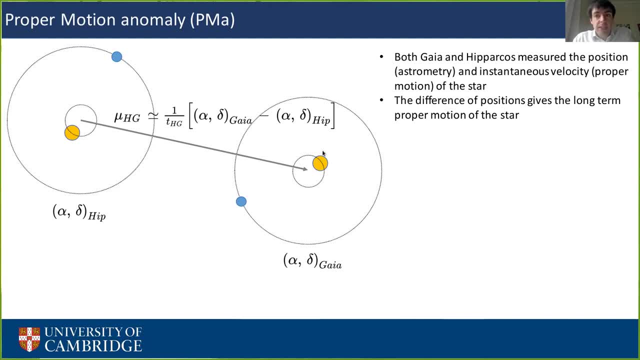 so if you take the astrometry of the stars obtained by gaia, you subtract the astrometry from hipparchus and you divide by the time between the two, which is about 35 years, then you get a measurement of the proper motion, uh, the long-term proper motion of the system. 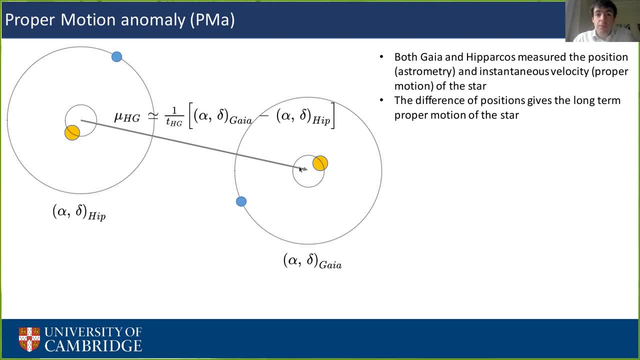 so the velocity, basically of the of the system of the sky. now, that's not the only measurement you have. if you look at the gaia data, you also have a measurement of the um, say, instantaneous proper motion, and this instantaneous proper motion is actually a combination of the long-term proper motion which i call here mu star. 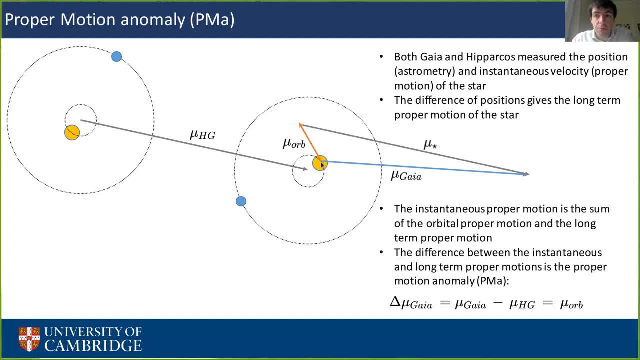 and the reflex motion or the orbital proper motion, the orbital motion of the star. so if you take this instantaneous measurement made for example by gaia, and you subtract the long-term proper motion which you get from the difference between the two catalysts, then in principle you should: 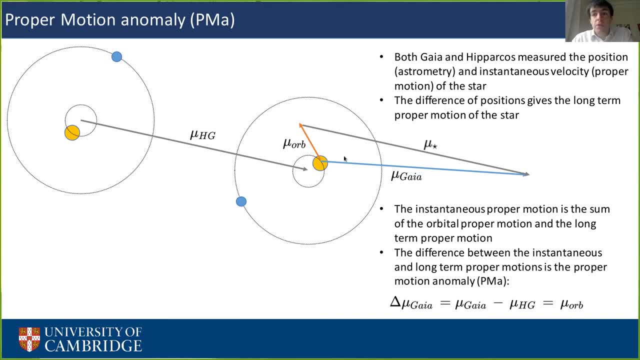 have a measurement of the orbital component of the motion and this quantity, the difference between the instantaneous motion and the long-term proper motion, is what we call the proper motion anomaly. so if you have a planet without a planet, then the instantaneous proper motion and the long-term 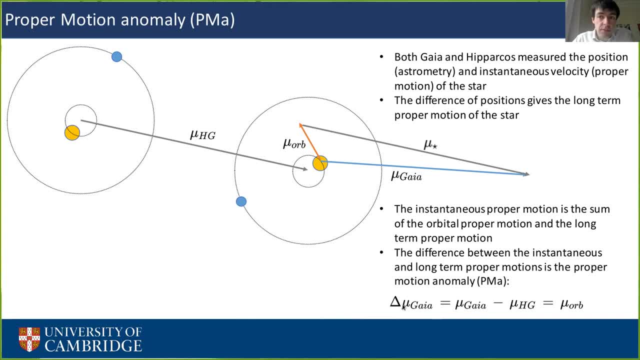 proper motion should be equal and this quantity- the proper motion anomaly, should be zero, whereas if you have a planet or another companion orbiting around the star, you should see this as a proper motion anomaly. now you can calculate a proper motion anomaly at the gaia epoch using the: 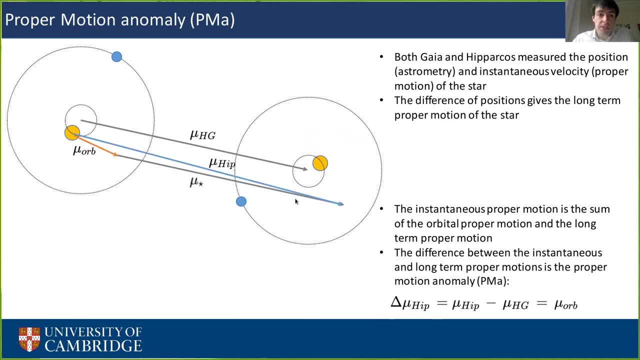 gaia instantaneous proper motion. you can also, of course, calculate the proper motion anomaly at the hypocholous epoch, and then you would get a proper motion anomaly at the hypocholous epoch, and then from this you can start to look for companions to stars. 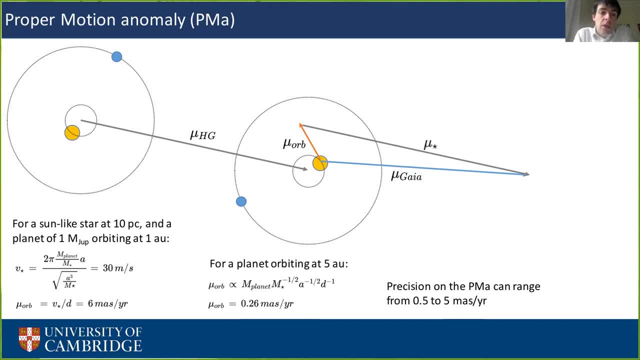 so if you look at the order of magnitudes, if you take a sun-like star at 10 parsec and a planet of one jupiter mass orbiting at one strom per unit, then the typical velocity, the orbital velocity of the star, is going to be so that it is in the order of magnitude of the star which is going to be. 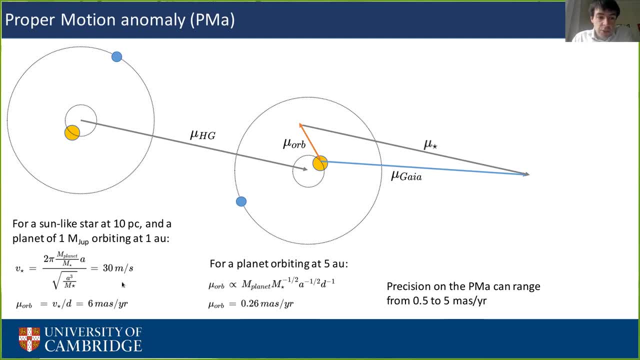 something like 30 meters per second, which translates to 6 milli arc second per year, on the sky at a distance of 10 parsec. if you take the orbits face on, if you go to five astronomical units, then you have something which is more like 0.26 milli arc second p. now this, this motion. 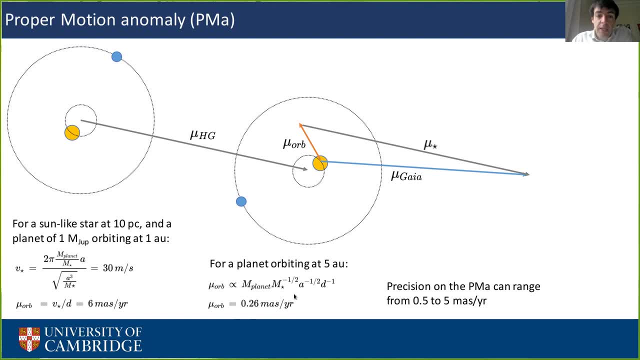 because its orbital motion scales as the mass of the planet, the inverse of the square root of the mass of the star. so it's easier to look for planets around small stars with this method. it's also scales as the inverse of the square root of the separation. 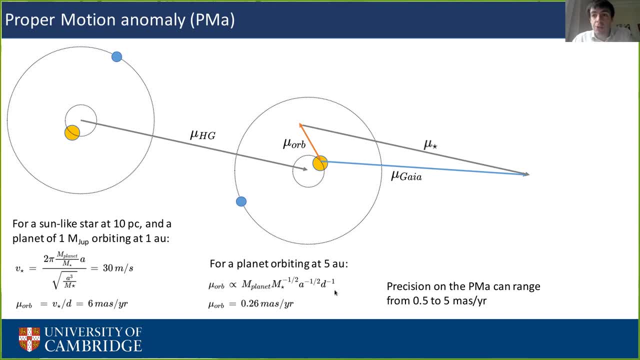 and of course the inverse of the distance, simply because of the geometrical projection. but then if you look at the catalog and and you do the the calculations, then the typical precision in dr2- actually i don't know in dr3, but the typical precision on the proper- 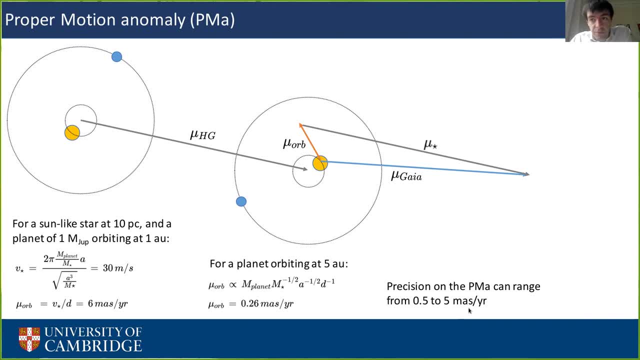 motion normally depends on the targets. depends on many different factors, but it can range anywhere from 0.5 to 5 milli arc second per year, typically. on some targets it's even better than this. of some other targets it's worse, but that that's the typical ballpark. 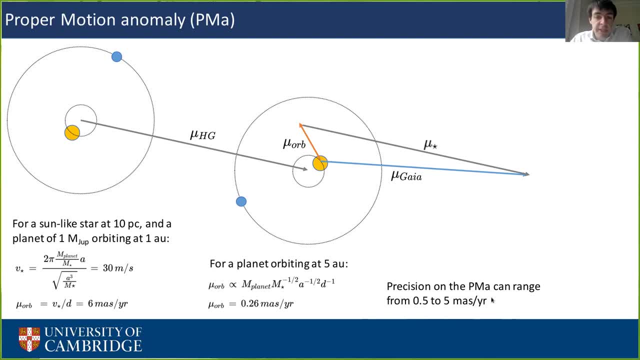 which means that with a method like this, basically we can expect to find planets of, say, a jupiter mass. that's the typical order of magnitude, maybe a bit more if the star is close to the sun, then we can hope to find less massive planets, but that's, that's the typical. 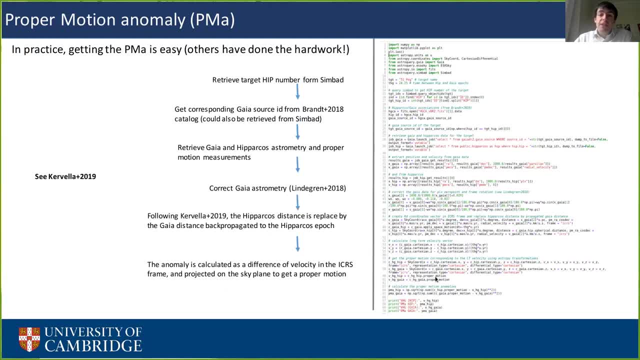 order of magnitude now. so i did the um, the exercise to prepare this, this presentation. i used a, a paper which is dedicated to this idea. it's paper by kabyline colleagues in 2019- and i tried to work to reproduce some of the results. so, basically, 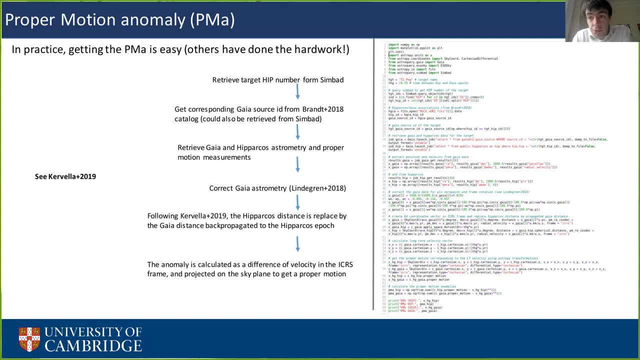 my question was: how hard is it to uh to do this, to do this, to use the hypocrisy and the gaia data to try to find uh, calculate proper motion anomalies and find planets? and the answer is um, it's actually not very difficult, and i think one of the reasons for 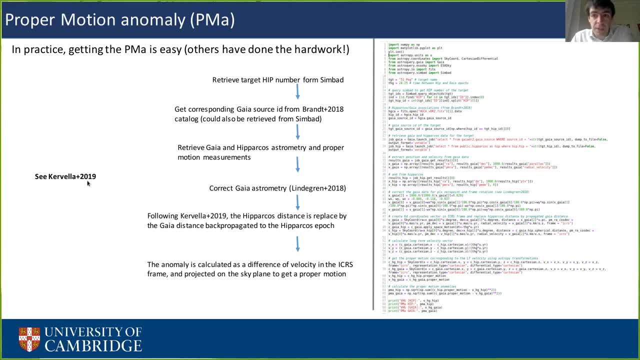 this is, uh, where, of course, first, other people have done that before, so i basically, in my case, i just followed the recipe pretty much, but also, um, other people have done the hard work. actually, if you look at the and the gaia and hipparchus catalogs, those catalogs are very 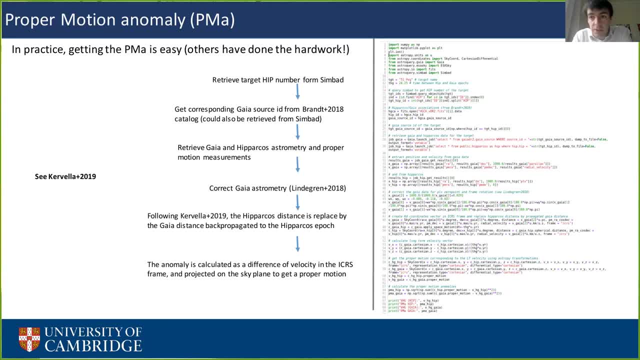 easy to use because other people have the whole data reduction and all the difficult work. so if you want to get a proper motion, normally the recipe goes like this: typically you take your targets. so uh 51 peg- that's my target. you get the hipparchus number from uh simbad, for example, so you can. 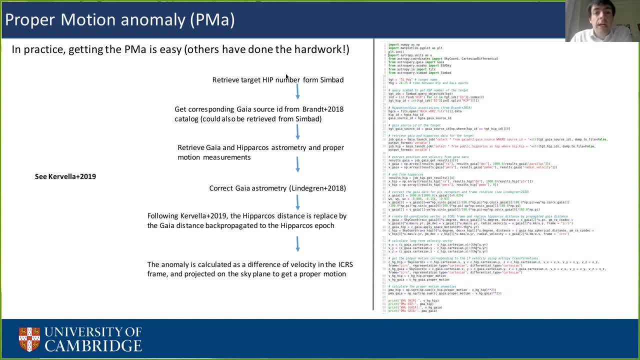 easily do this in python using, for example, astroquery. so you get the hipparchus number and then you need a way to get the corresponding uh gaia id number. so i think there's a number of ways to do this. um, i think you can even get the gaia id from simbad, but in my case i used a catalog. 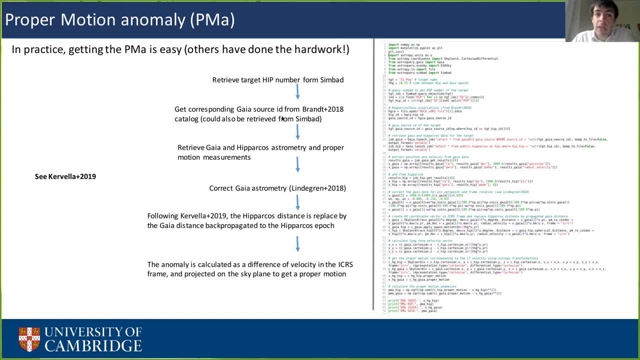 i learned in colleagues in in 2018 uh where you have the cross correlation between the parkers and gaia. so from the hipparchus uh id number i could get the gaia id number. then once you have the two uh ids of your targets in the two catalogs, then you can query the two catalogs. 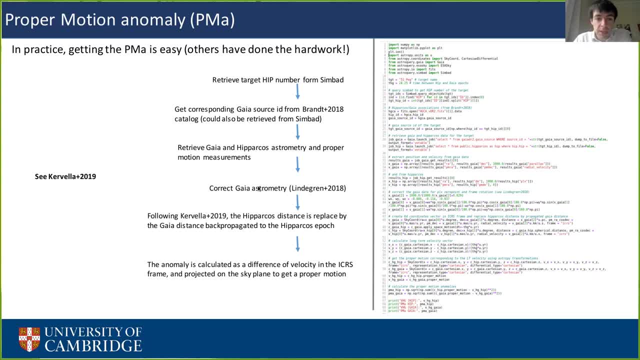 you get the astrometry and proper motion at the two epochs, then there's a little bit of cooking, at least for dr2, um gaia dr2. there's a little bit of cooking to um correct the uh gaia data, but it's not very difficult. then you can play a little bit with the. 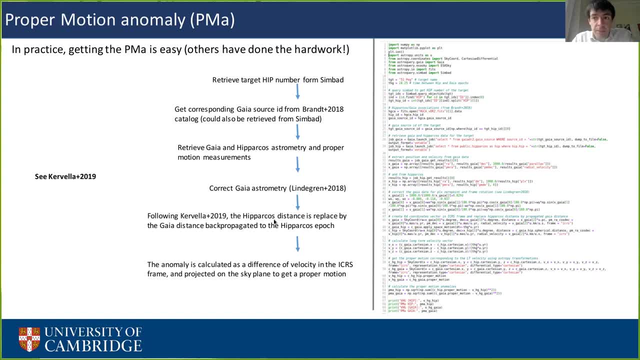 parallax. the parallax from gaia is much better than the parallax from the parkers, so you can- basically you can- back propagate the gaia distance using radio velocity data to the parker's epoch and replace the parker's parallax by this. 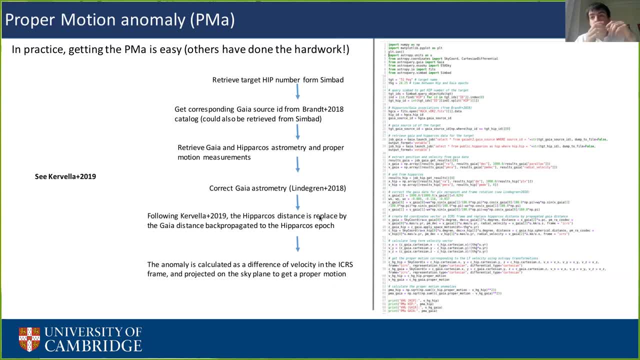 uh number can be important because of of the, the geometrical projection of the velocity of the star uh, which changes depending on the, on the distance, and once you have all this, then you can calculate uh, basically the velocity vector of the star, in the icrs frame, and then you project this on the 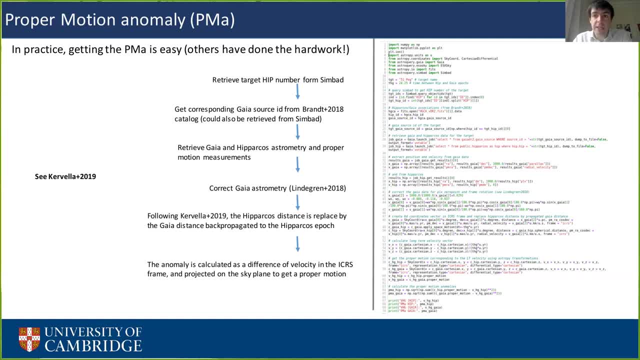 sky, uh, to get rid of the proper motion. so you project this at the reference epoch of hipparchus, at the reference epoch of gaia, and then you can calculate the proper motion anomaly. so it's yeah, basically you can do this in less than 70 lines of code. then you get. 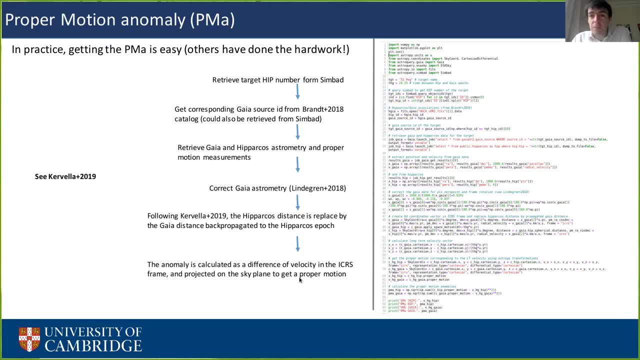 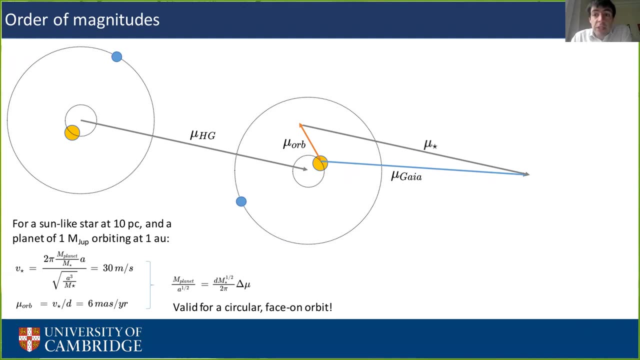 so it's not. yeah, it's probably not paper grade results, but it's, it works and you can get proper motion anomaly measurements or something like this. so relatively straightforward. so once you have a proper motion anomaly measurement, uh, what can you say about the, about the planet? so, actually, so i've shown that the, the proper motion anomaly, is um. 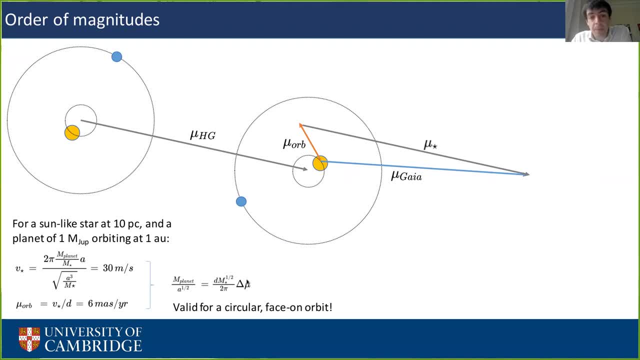 so if you know the mass of the star and you know the distance, and you do have the distance actually, at least from the, from the gaia data, so if you know this, then the proper motion anomaly is actually a measurement of the mass of the planet divided by the square root of the semi-major axis. 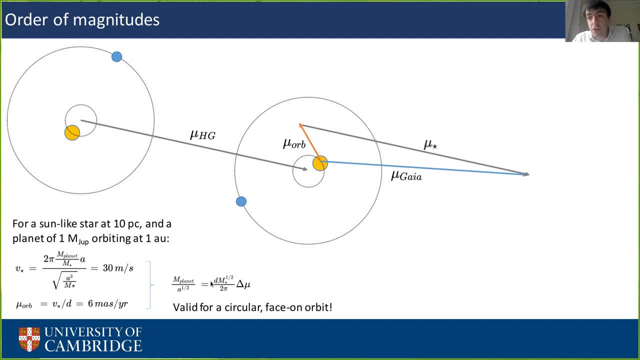 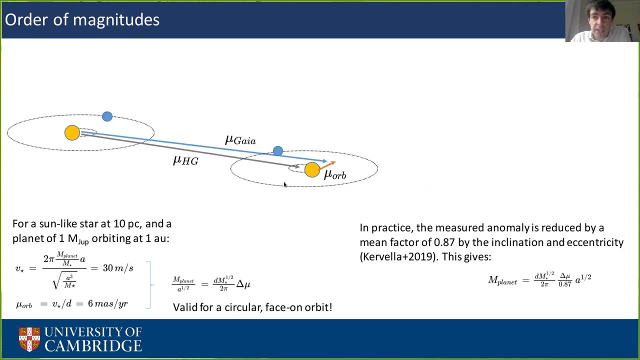 this is valid for a circular phase on orbit. if the orbit is inclined or if you have some eccentricity, then this isn't really true and you take this into account. so then it depends on on what you're doing from a statistical point of view, you can expect the inclination, the eccentricity and all of this. 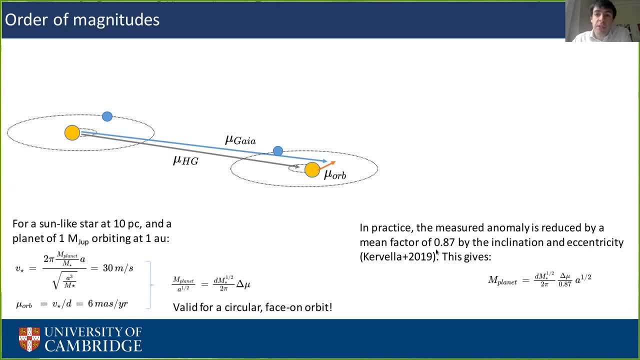 to reduce your measurement typically by a factor of 0.87, which means that if you're interested in the in the statistics of the proper motion, normally on many different targets, you can pretty much just multiply your your measurement by 1 divided by 0.87, and you'll get a decent result. if you're. 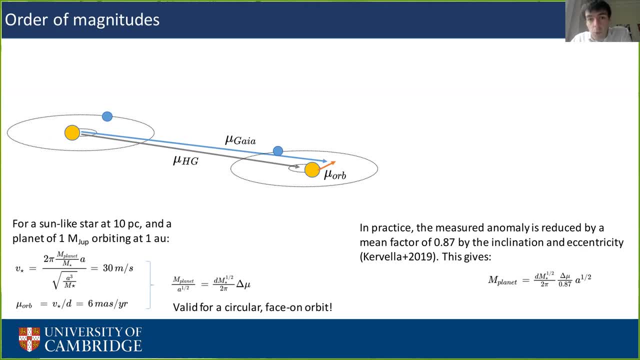 interested in one particular target, then you need some way to be able to take into account the true inclination, and i'm going to talk about this later on, but that that's the idea. so once you have this in principle, you have a measurement of the mass of the planet divided by the square root of the 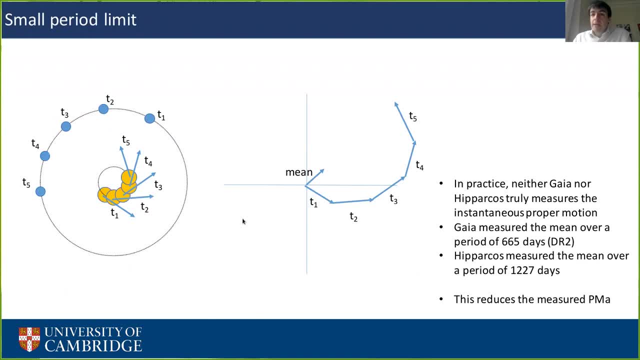 semi-major axis and you measure the mass of the model by looking at the other side of the graph. then what you're doing is you measure the mass of the model by using the range of the data you have and giving it the same number of steps of the graph. 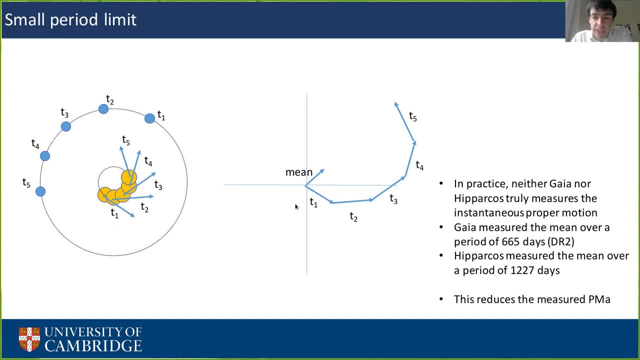 now it's not as easy because there are a number of r2 over 665 days and hypochors over 12, a bit more than 1200 days, and the problem with this, of course, is if you have a small period planet, so our planet, orbiting with a period which is 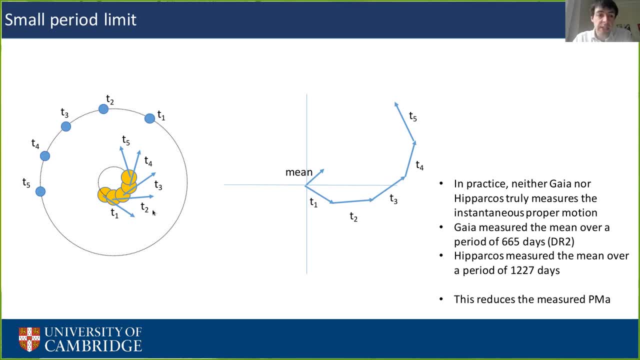 smaller than typically 665 days for Gaia. then averaging the measurement of the velocity at different times changes the result. it decreases the measured velocity simply because this velocity vector is rotating with time. so if you add all of this and you divide by the number of measurements, 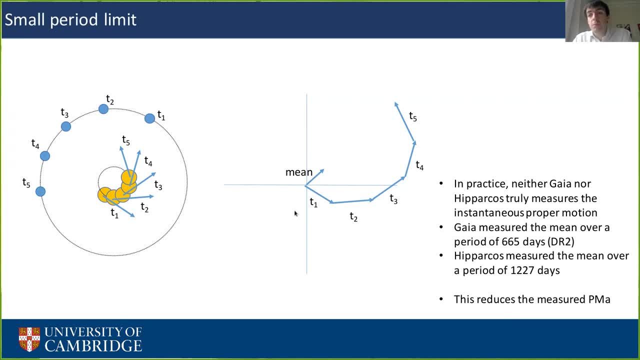 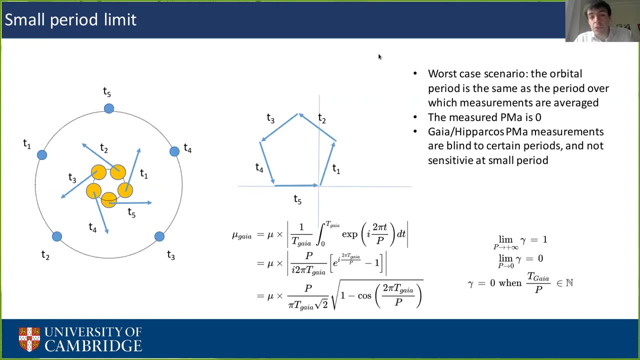 then the length of the proper motion you're measuring is going to be different from the true length of each of those vectors, simply because you're averaging velocity vectors which aren't linear to each other. so you can do the calculation. if you're interested, you can do the. 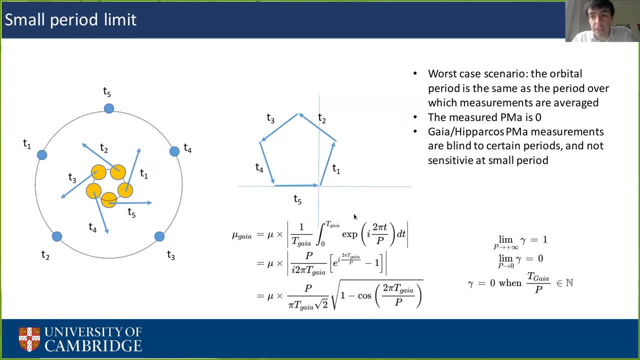 calculation to see what is going to be the impact of this on the, on your measurement, and you will find that the measurement you're doing is the true value of this orbital motion multiplied by a quantity which is like this: it's sometimes called gamma. it's the period, the period of the planet. 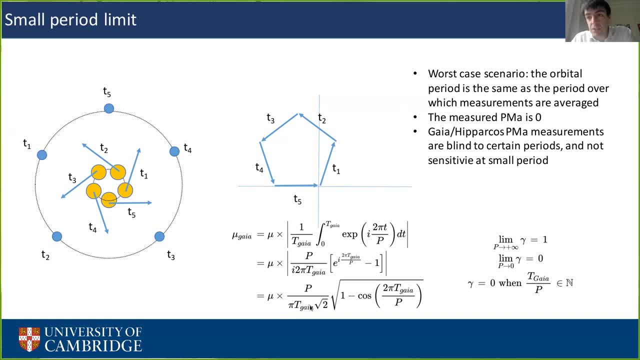 divided by pi times t Gaia, which is six hundred and sixty-five days times square root of two, all of this times the square root of one minus the cosine of two pi t Gaia divided by p. and if you look at this quantity here you can see several things. so first, this goes to one when p goes to infinity. 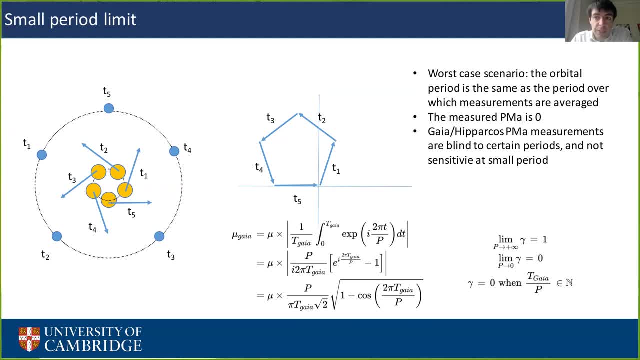 and you can expect this because the, so the. if you take a long period planets, you can expect that the averaging the data over a small window compared to the orbit of the planet isn't going to change anything. now, if you look at what happens for p goes to zero, so for very small orbital periods, then this quantity goes to zero. 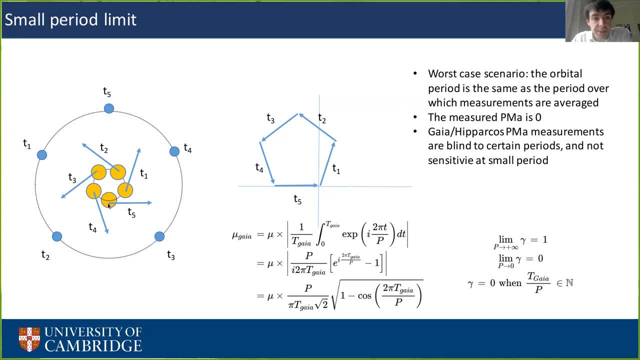 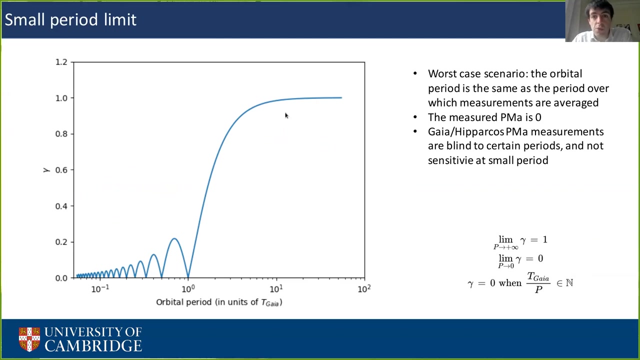 which means that, basically, if you take a small period and you average your measurements, your measurements, the data, and you're having a very long period, then you'll end up with like a very short period of time of the cycle, and so part of this equation is that the so this method isn't sensitive to small period planets, and then in between you have a bunch of zero when the 665 days from the observing windows divided by the period of the planet is an integer. so if you prop this function, uh, you get something which is uh, like this: so it goes to zero for small period was to one for long period planets and in between you have a bunch of oscillations. 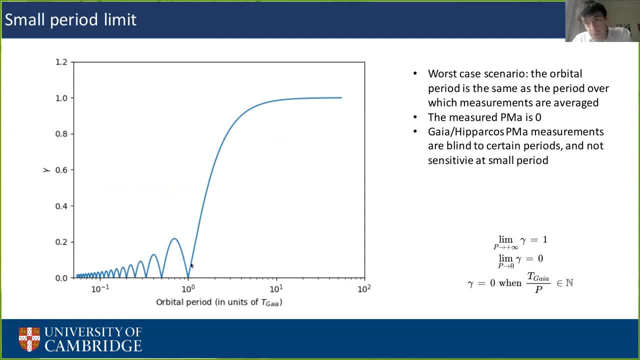 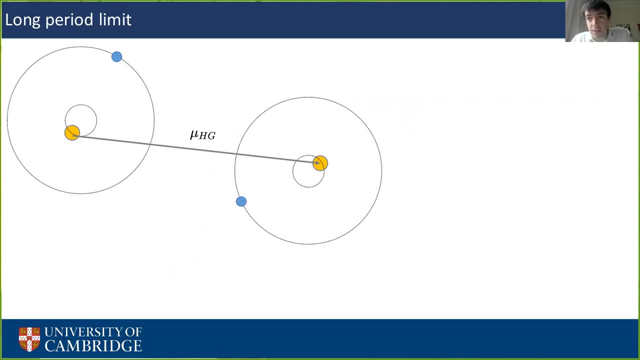 So that's a problem for small period planets. You can't really detect them with something like this If you look at the other extreme for long period planets. so this observing window smearing doesn't really impact long period planets, but you have another effect that you need to take into account. 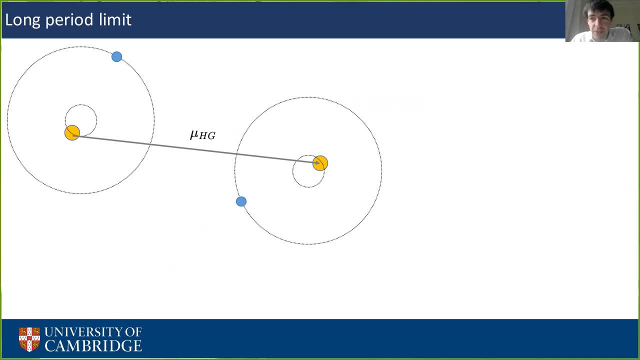 which is that you don't truly measure the proper motion of the star with Hipparchus or Gaia, but you also don't really measure the long term motion, because what you really measure is the position of the star at the Hipparchus epoch and at the Gaia epoch. 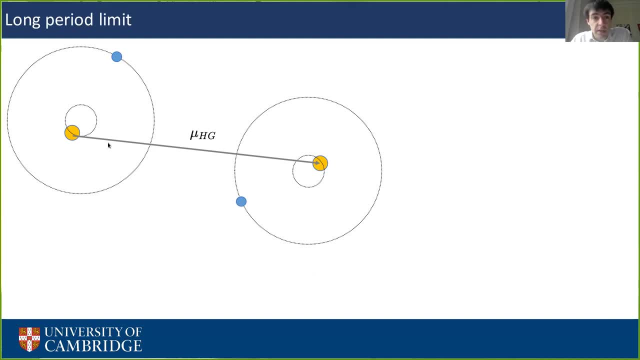 But then this motion of the star is already a combination of the proper motion of the system and the orbital motion of the system. So if the orbital period is small then it doesn't really matter. But if the orbit has a long period then it's actually very difficult to separate the long term proper motion of the star from this long orbital motion. 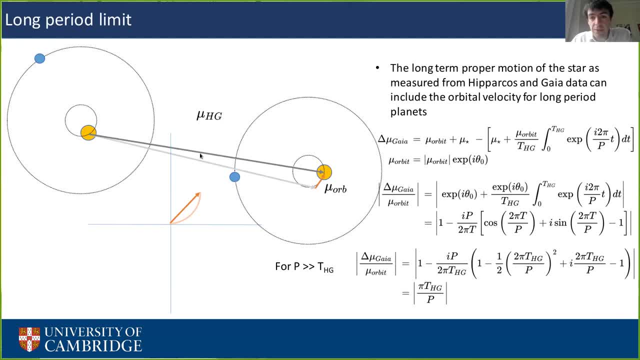 this long period orbital motion, And again, you can do the math if you're interested, at least for a circular phase on orbit. It's not very difficult to do And you would find that for long period planets, this anomaly measured with Gaia divided by the true value of the orbital motion, 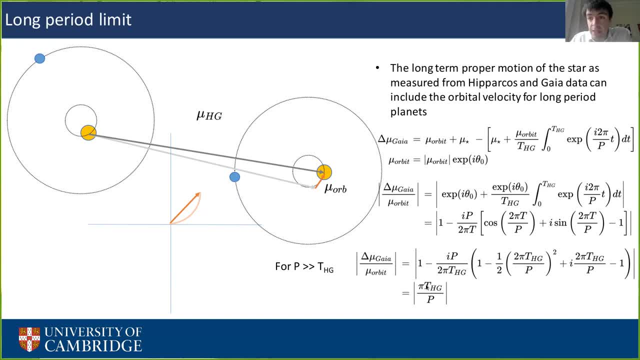 is something like pi times the time between Hipparchus and Gaia, so about 45 years divided by the orbital period. And so that's true in the long period regime, And in between you have to do a proper calculation which you can do numerically. 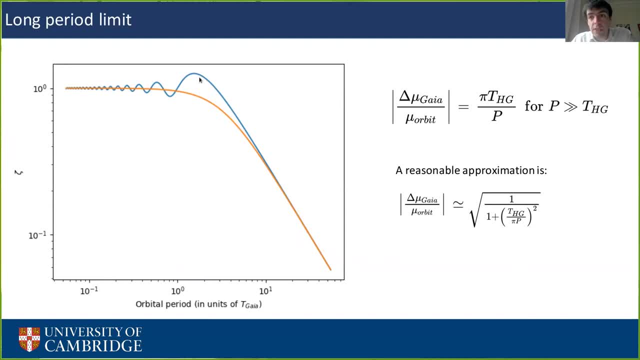 And you would find something like this, something like the blue curve for the proper calculation, And you can approximate this with a formula like this and you would get the orange curve. And what you see here is for this effect. it doesn't really change anything for small period planets. 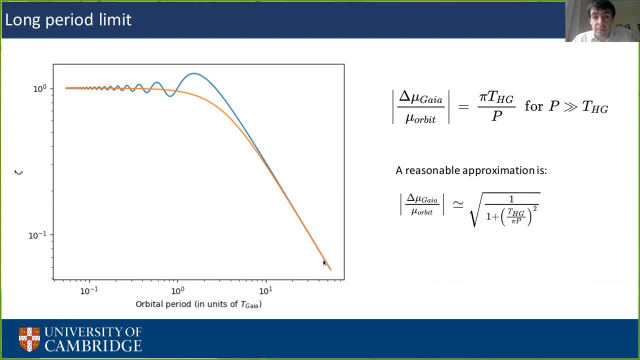 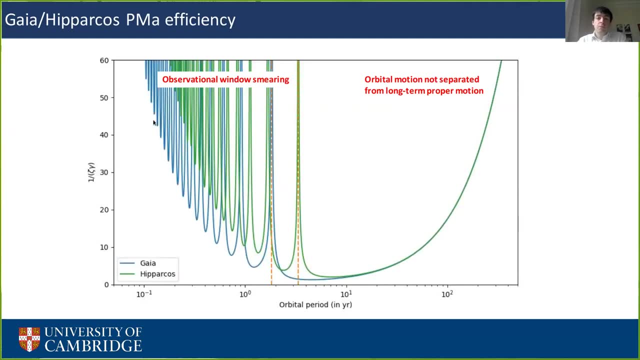 But it does reduce the sensitivity of the method at long periods, And so if you combine the two phenomena, you can plot something like this, which would be the sensitivity of this method, And you would see that basically, so you're not really sensitive to long period planets. 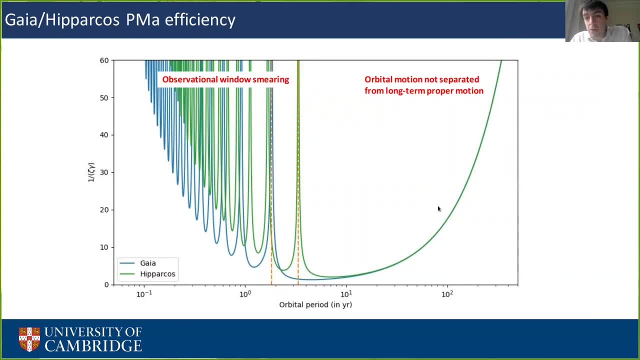 because of this problem of separating the long time of motion from the long period orbital motion, And you're not sensitive to small period planets because of this observation of the Windrush mirror. So this method is typically sensitive to planets orbiting with orbital periods of. 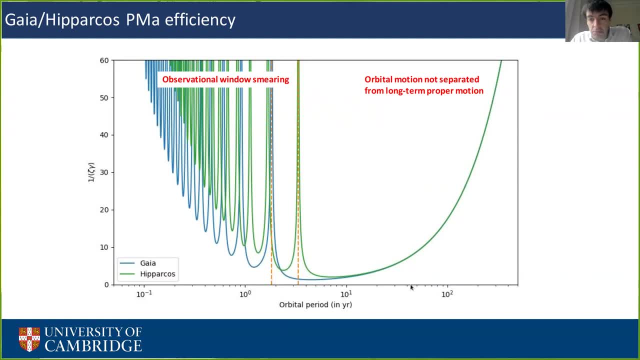 say from one year maybe to 30,, 40,, 50 years. So that's the typical range of orbital periods at which this method is sensitive. Then in blue you have the sensitivity for Gaia, And so for the Gaia proper motion anomaly. 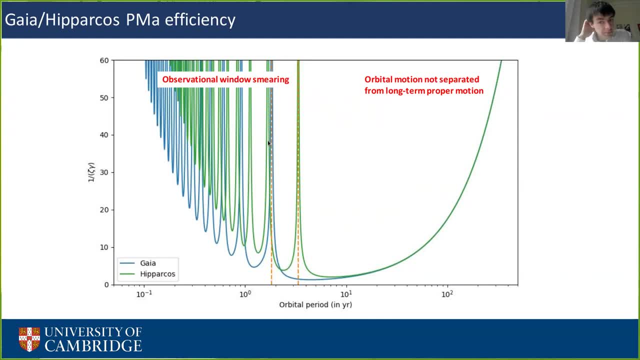 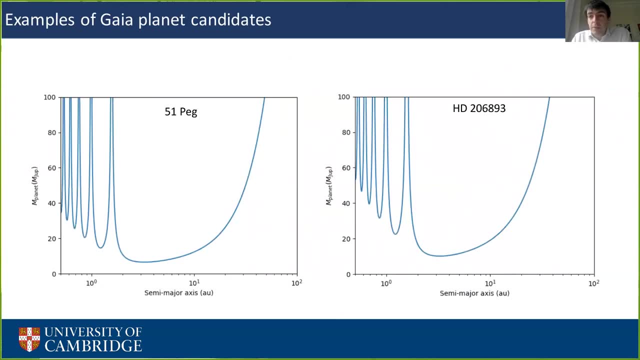 And in green for the Pythagoras proper motion anomaly. So if you do this, if you get the data from the Hipparchus and Gaia catalogue after the proper motion anomaly, then take those effects into account. you can do something like this. 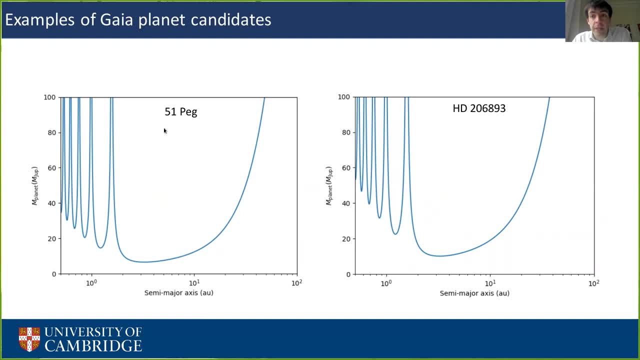 which would be so, for example, for 51 Peg you would find a proper motion anomaly- I don't remember what the value is, but you'd find a proper motion anomaly for the star- And then this would be the mass of the planet as a function of the semi-major axis. 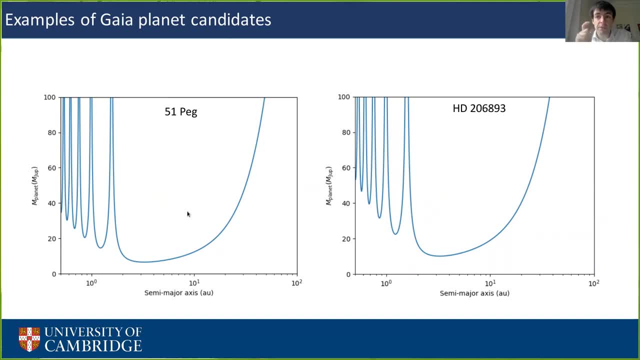 which we needed to explain this level of proper motion anomaly, And I've also plotted this for another star, HD 206893.. I'm going to talk a bit more about this example later on, But so again, you see that the typical range 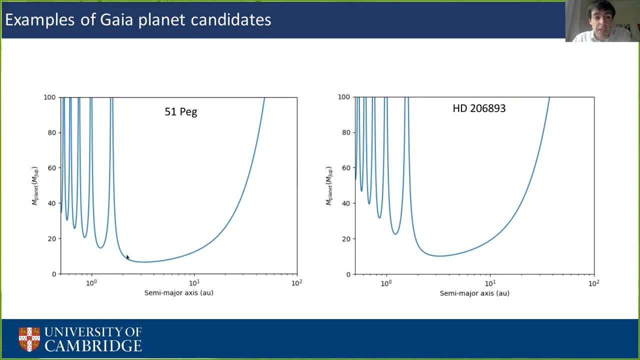 of semi-major axis at which you're sensitive is typically a few astronomical units to 10, 20 astronomical units. That's the typical ballpark, And then you get to masses of maybe a few Jupiter masses can be less than that for stars. 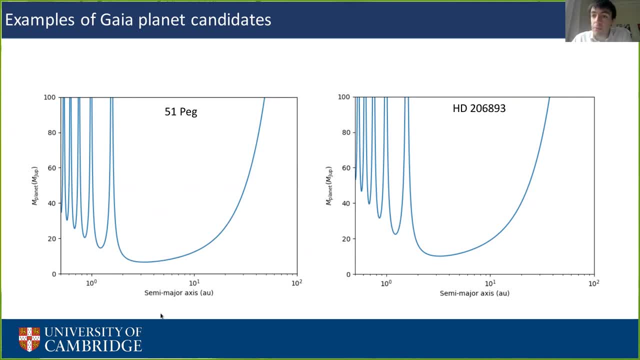 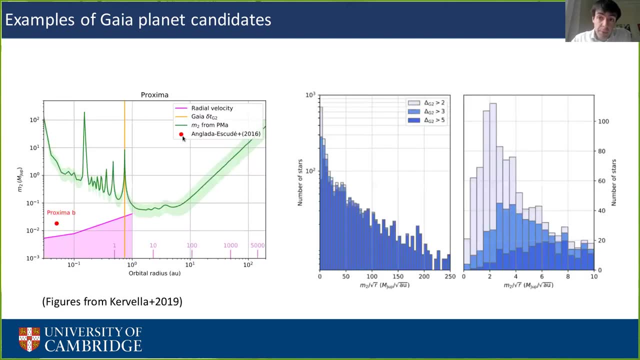 which are not too far away from our Sun, But that's the range of planets that you can expect to detect with this. Now there are a number of refinements to the method, especially for stars which are close to our Sun because of many geometrical effects. 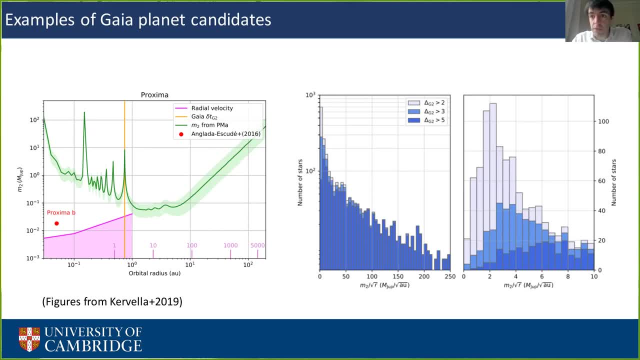 that you need to take into account, But you can also do this, for it works very well for stars which aren't too far away, And this is an example figure which I took from Kavala and colleagues: 2019 for Proxima. 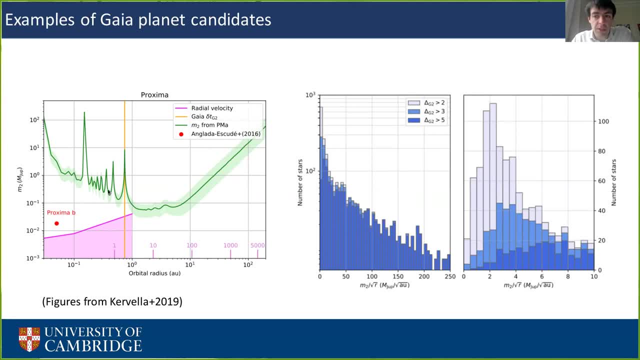 So again the same idea: proper motion anomaly is detected around Proxima, And in this case it's a close by star, which means that the range of mass to which the method is sensitive goes below one Jupiter mass. And so you see the mass. 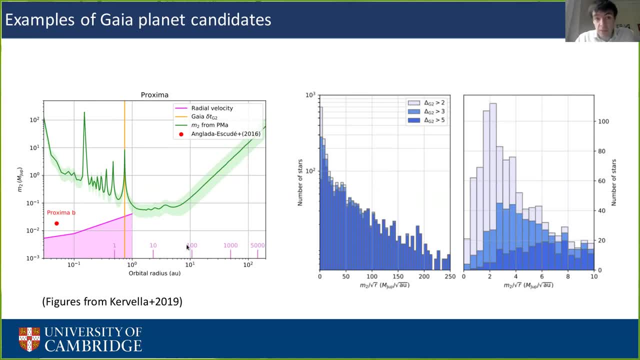 as a function of the orbital ranges needed to explain the proper motion anomaly of Proxima. And you see that Plan B actually cannot explain this proper motion anomaly. So of course this is related to Proxima C, which I'm going to talk about again just after this. 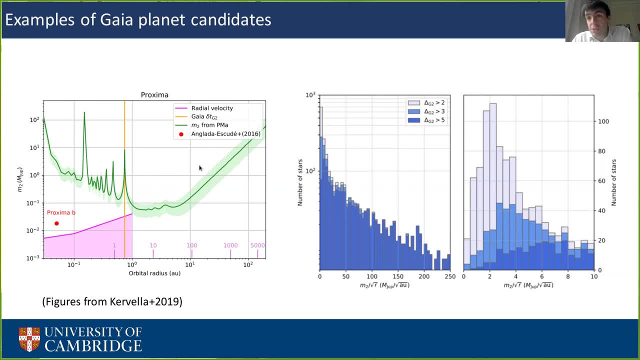 So that would be a way to study some particular targets And if you're interested in one target then you can get the proper motion anomaly and work with it. You can also look at what happens statistically If you look at all the data in the Hippogus catalog. 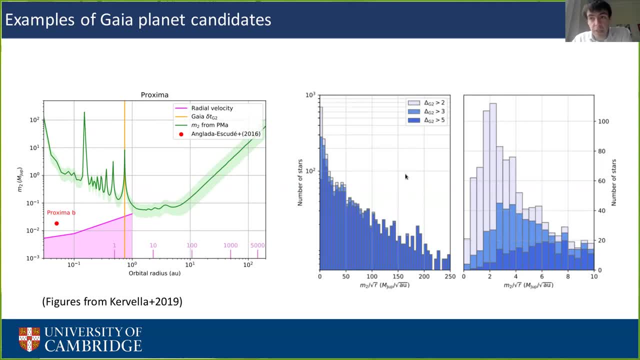 and the Gaia catalog. how many planet candidates can you find? And this is again a figure taken from this paper, the same paper which gives the number of stars around which there is a proper motion anomaly which translates to a given mass divided by the square root of the radius. 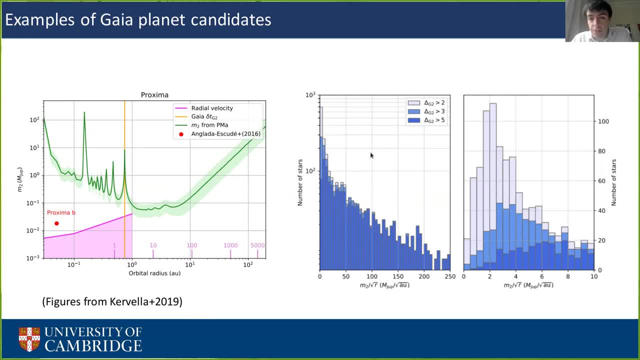 for different confidence levels- five, three and two. And if you take this and you zoom at the range of masses that we are really interested in today, because we're talking about exoplanet detection, then you see that the number of candidates. 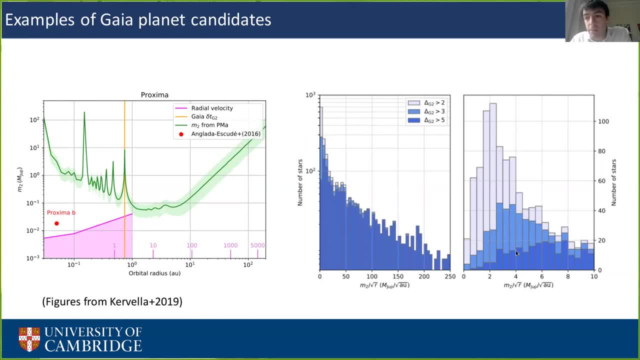 you have from those catalogs is typically a couple of hundreds for a confidence level of five, And if you go down to a confidence level of two in the light blue here you have a few hundred candidates. So that's typically what you get with the proper motion. anomaly observations. 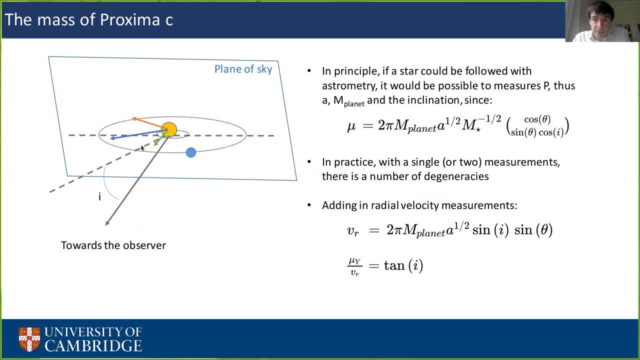 Now again, if you're interested in a particular target, it's not as easy, because then you need to take into account the fact that the orbit can be more complicated than a circular phase. on orbit You can have possibly eccentricity, which I'm not really going to discuss. 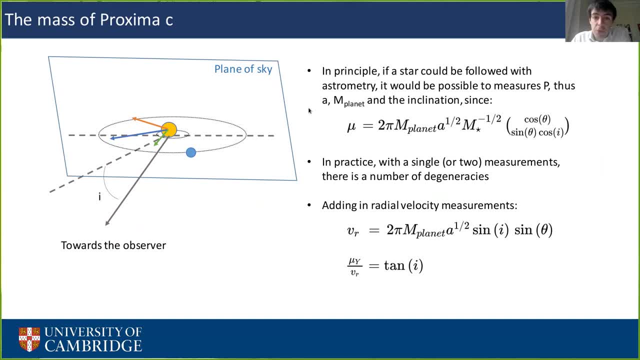 but you can have, of course, an inclination of the orbit, So you don't really So in principle. if you could follow the star and get many measurements of the proper motion anomaly, which would translate in many measurements of the orbital motion of the star, 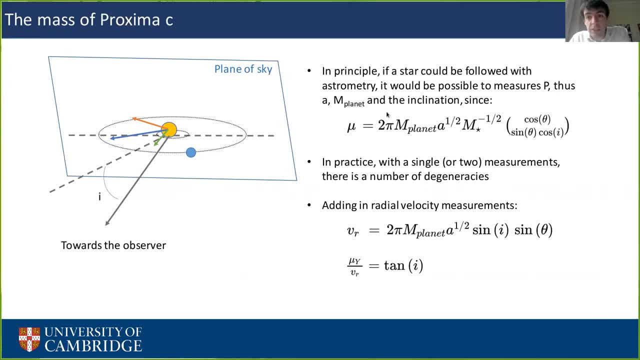 you could basically reconstruct the orbits and you would be able to measure the inclination, the eccentricity and the true mass of the planet and the semi-major axis, basically everything. The problem is, in practice. you don't have many measurements. 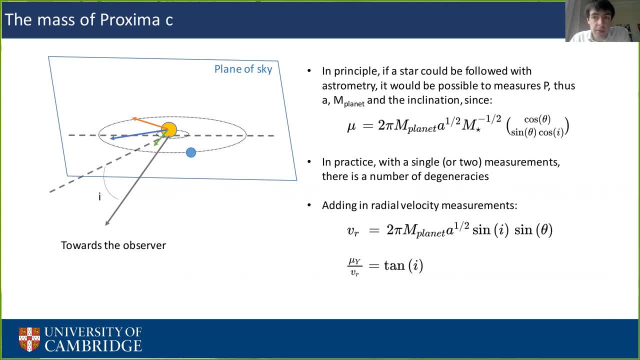 You only have one or two, if you have the two epochs, the Apocrypha and Gaia, but you don't have anything more And with this you cannot actually get a measurement of the orbit at the point of the true mass of the planet. 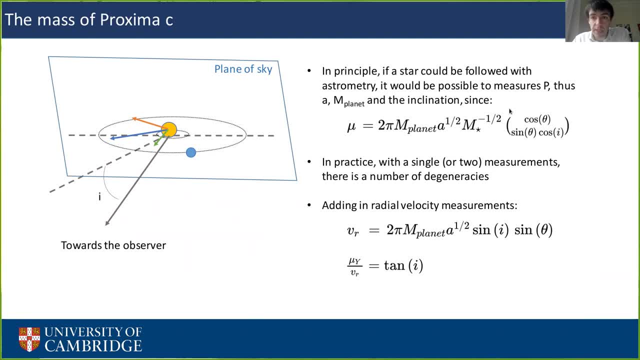 because you have a generality with the inclination and also with the orbital phase. So there are a number of ways to go on this. One of them is to add radial velocity measurements. If you also have radial velocity measurements, then basically you have a measurement of those. 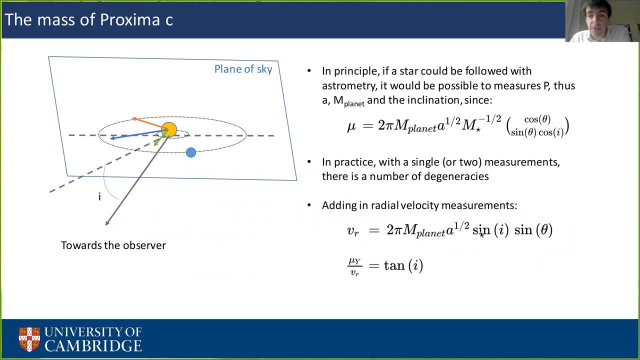 So first you have a measurement of the mass of the planet times the sine of the inclination. You also have the orbital period and you also have the orbital phase from the radial velocity curve. So if you combine this with the proper motion measurement, then you can get the inclination of the planet. 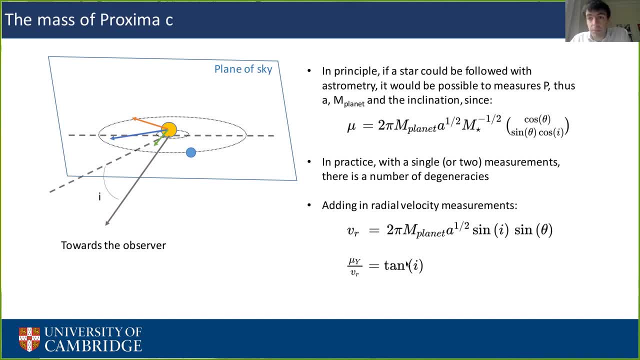 And once you have the inclination, of course, you can get the true mass of the planet. So this is a really powerful combination. actually, Even if you have only one proper motion measurement, if you combine this with radial velocity data, you can still retrieve the inclination and the mass. 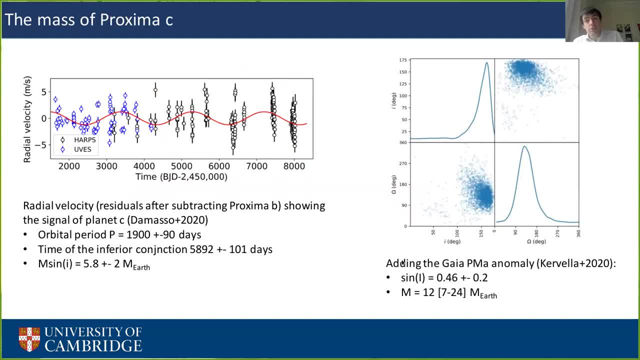 And this is something which has been done on Proxima C actually. So this is a plot which I took from a paper by Damaso and colleagues in 2020, so quite a recent paper- where you see the residuals of the radial velocity data. 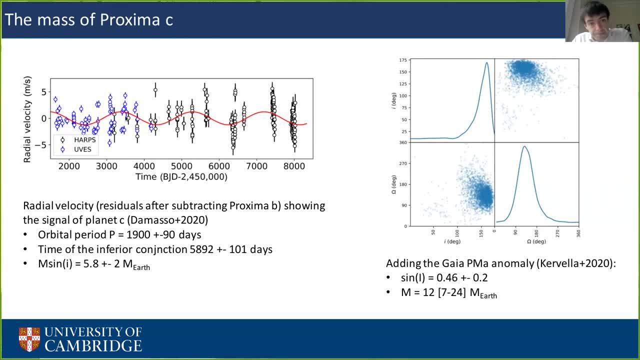 after the subtraction of the signal from Proxima B, And here you see the signal from Proxima C. Now, using radial velocity, you can, as I said, measure the orbital period, measure the possible time of the conjunction and the m-sine inclination. 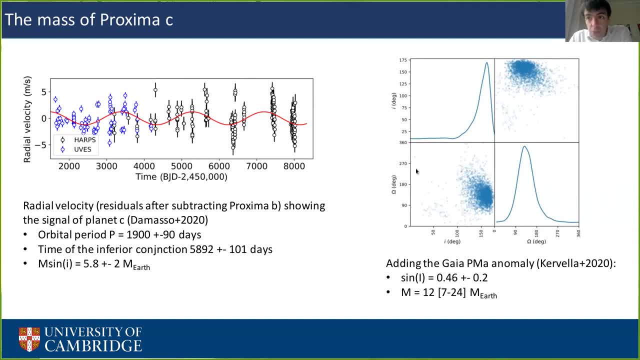 So if you take those measurements and you also add the proper motion anomaly, then this is something which has been done also in 2020, you can retrieve the value of the sign of the inclination and then, of course, of the true mass of the planet. 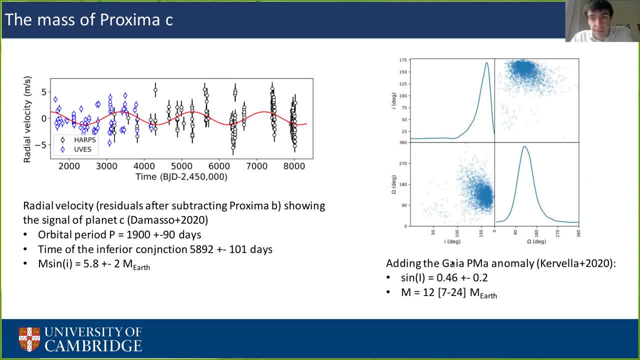 So a powerful combination. What is also, I think, very interesting is, once you have the sign of the inclination, then you start to have actually quite a number of measurements. You know the inclination, you know the period, so you know the semi-major axis. 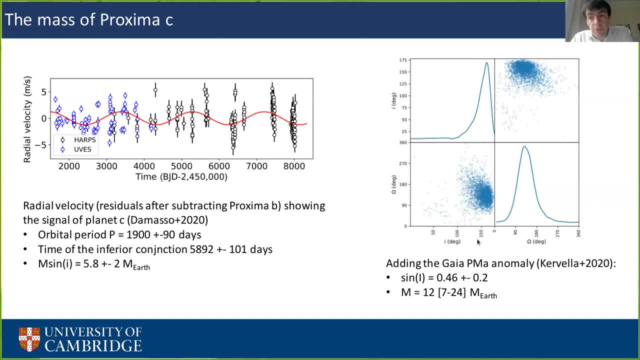 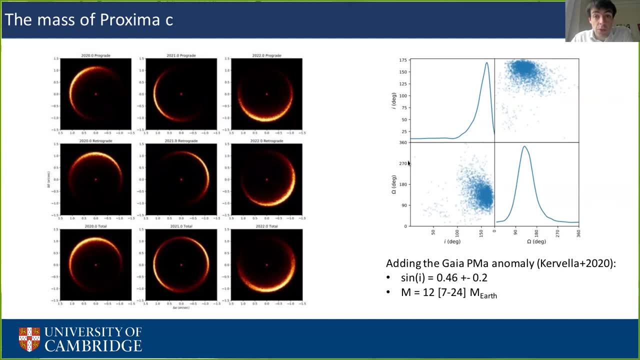 you know the orbital phase and if you combine all of this you can actually start to predict where the planet is around the star. So none of those methods- astrometry and radial velocity- is sensitive to the position of the planet. You're just looking at the star. 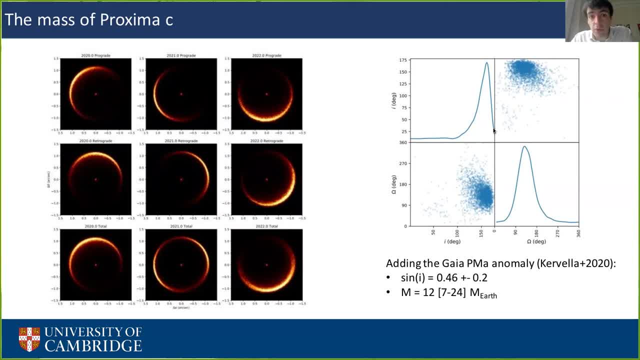 So in principle, you cannot say where the planet is, But if you combine all of this, you can actually start to have an idea. So this is again taken from Kavila and Pauli's 2020 prediction: the probability- 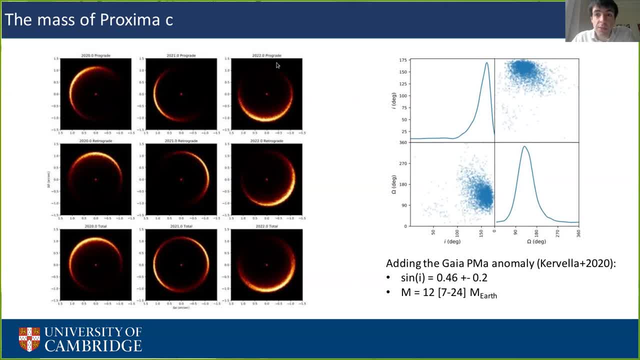 the probability of the presence of the planet at different epochs and in difference for different orbits, because basically you only have a measurement of the sign of the inclination, so you have two possible values in terms of inclination. But that gives you an idea of where the planet can be. 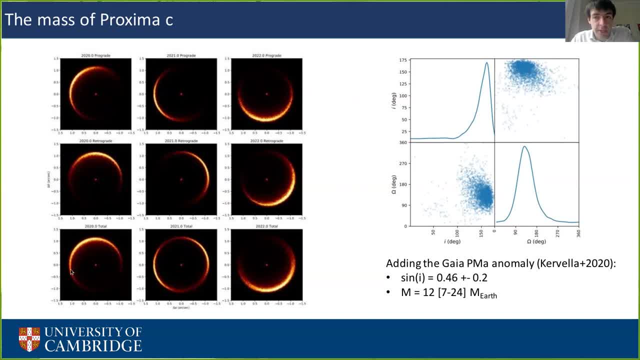 So in this case, unfortunately, you cannot really pinpoint the location of the planet, But I think that's an interesting first step towards being able to predict where the planet is in the sky only based on star measurements, radial velocity and proper motion. And again, 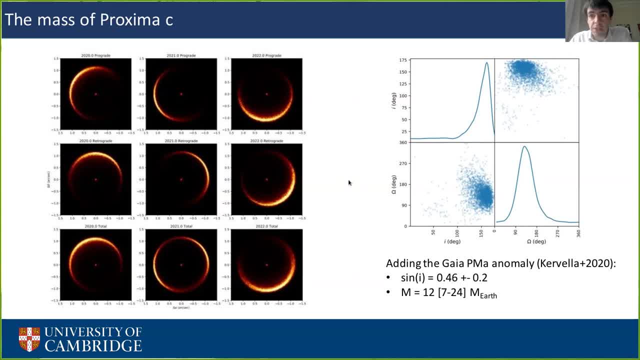 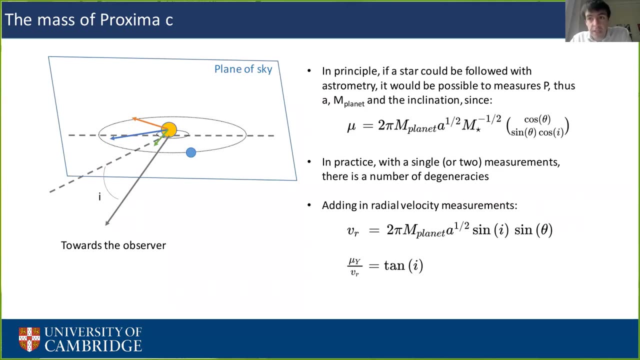 this is important, for example, for direct imaging or long baseline interferometry, where we need to know where the planet is if we want to observe. Now, if you don't have radial velocity measurements, for example, interested in a young target where radial velocity? 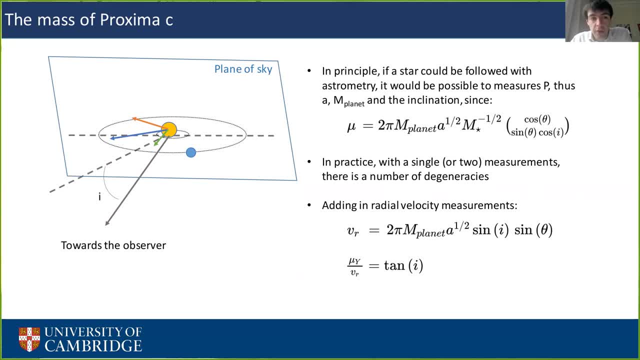 is very difficult to obtain properly, so you don't have radial velocity measurements. you can still do something if you have, for example, a direct detection of a planet in the system, Because if you have a direct detection of the planet, then basically you know. 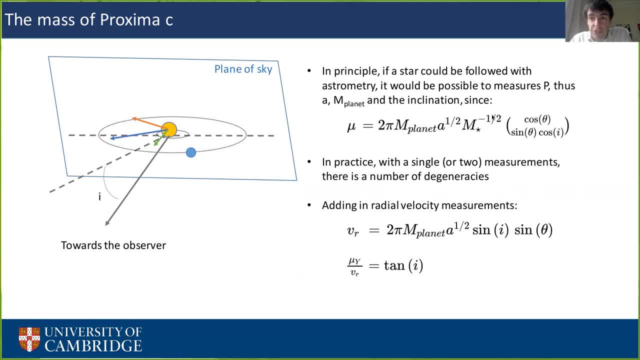 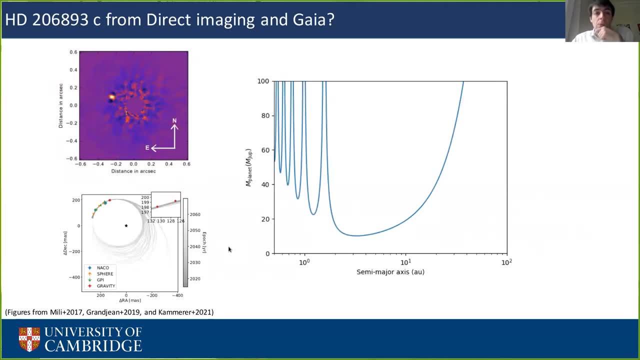 the orbital phase, So you can also break this degeneracy and get a measurement of the true mass of the planet. And I think an interesting example is HD 206893.. So this is a star around which there is one, at least one giant planet. 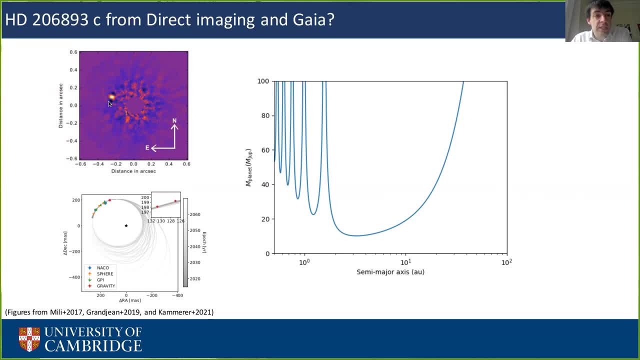 close to a brown dwarf, actually HD 206893 b, which has been observed with direct imaging And actually long baseline interferometry. we've observed this target with the exo-gravity large program. So this is an interesting example because, if you look, 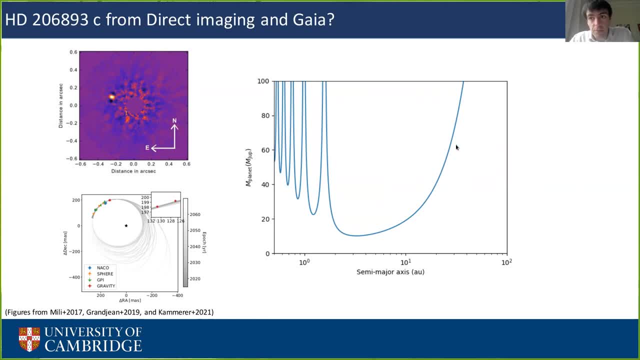 at the proper motion anomaly using what I've explained before, then for this target you would get a graph which is a little bit like this: And if you look at the mass of the, if you look at this planet, then typically you can explain. 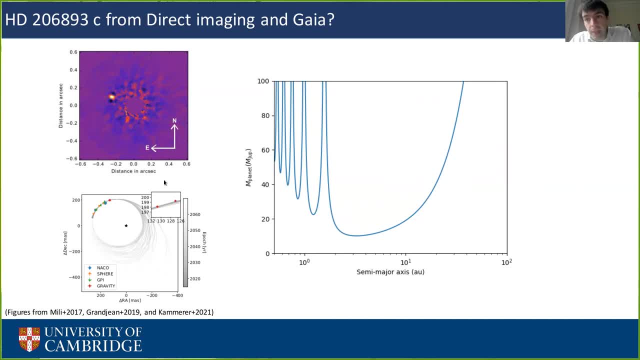 this proper motion anomaly, just with this planet b. Now this is if you look at the proper motion anomaly as a scalar quantity, So meaning you're just looking at the amplitude of this proper motion anomaly. Now, technically, when you measure the proper motion anomaly, 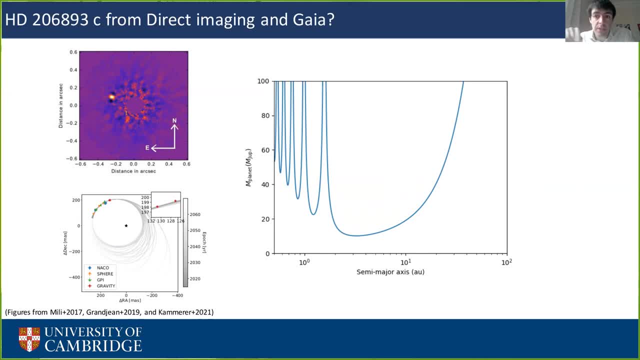 you don't have just a scalar quantity, you have a 2D vector on the scale, So you have a proper motion anomaly in alpha right ascension and declination. So it's a bit difficult to do this because you have to be very careful. 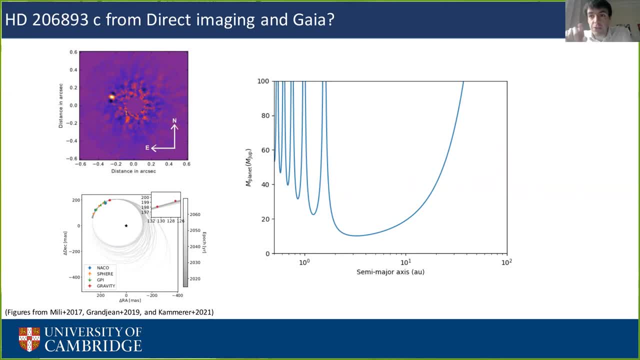 with this averaging of the measurements made with Gaia. So you have to take this into account. but you can get a 2D proper motion anomaly And in this case because we know where the planet is, because we have those direct imaging observations. 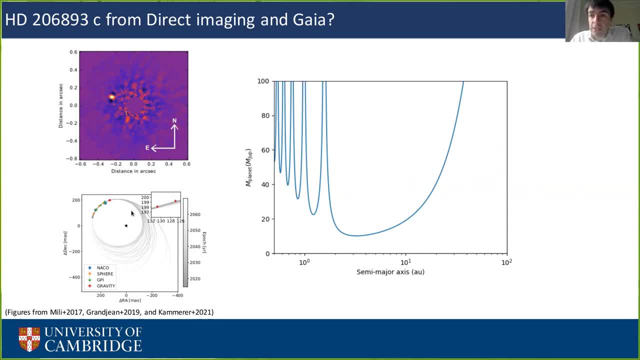 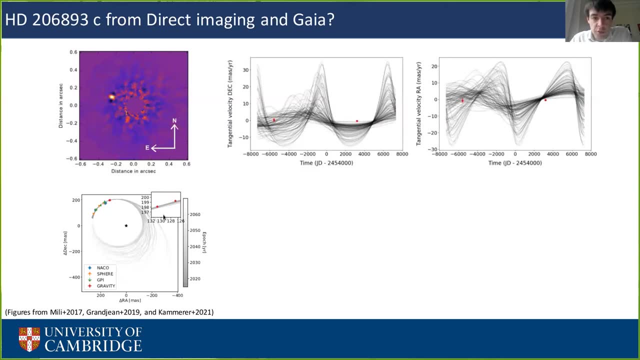 so we know the orbit, we know what should be the orientation of the proper motion anomaly. And if you look at the true orientation of the proper motion anomaly- those figures are taken from a number of papers which are listed here- then you see that the proper motion anomaly 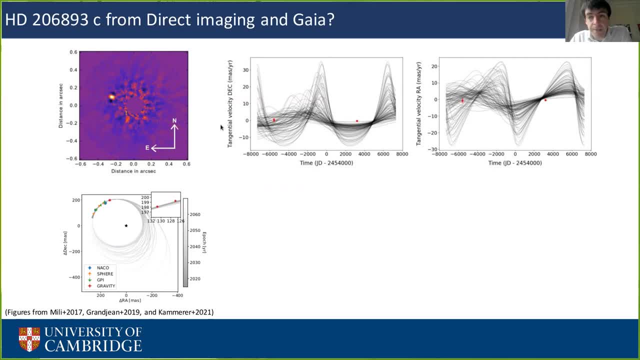 generated by this planet B cannot really explain the proper motion anomaly observed from Targus and Gaia. So you actually need another planet in the system to be able to explain this, And so a very recent paper by Jens Kammerer also looked into this. 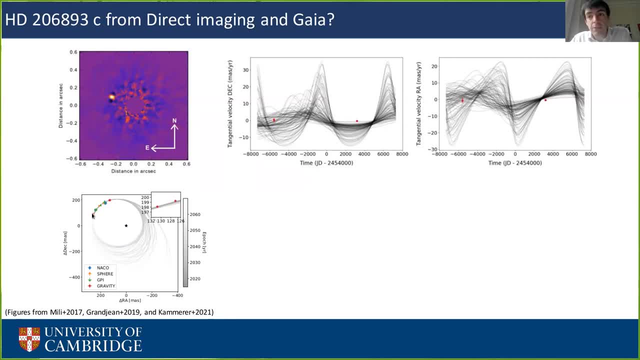 adding gravity observation of planet B, which are very helpful to get a much better orbit estimate. So if you have a good orbit estimate and you have those measurements, then you can actually start to sort of predict where this planet B- planet C, sorry- should be on the sky. 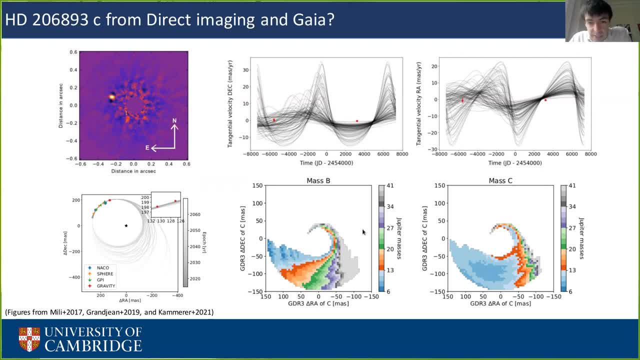 And you can even draw plots like this where you have the mass that you need for planet B and planet C, depending on the location of planet C, to explain the proper motion anomaly. So you can start to have sort of an idea of what is going to be. 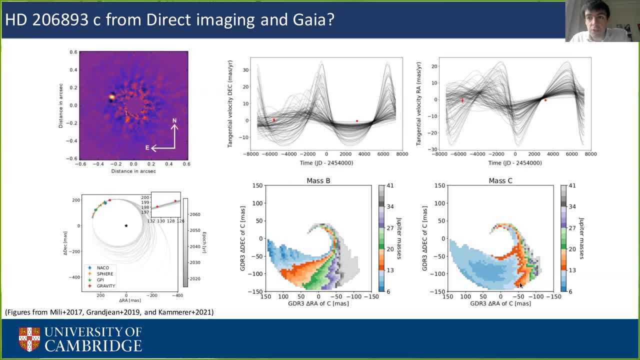 the mass of B and the mass of C and the location of the two planets just from this combination of direct observations of B only, not C, and proper motion anomaly. So a very interesting way to start to detect unseen planets around stars or on which we already have another planet. 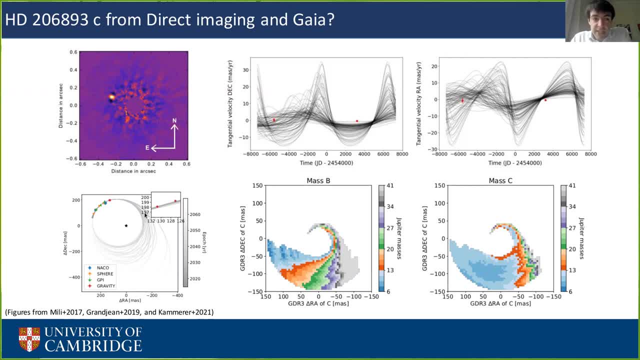 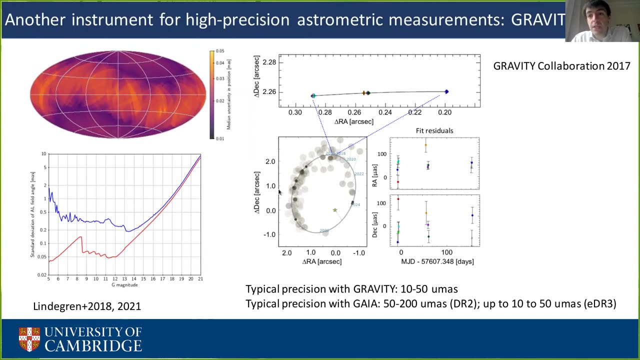 So I said that in this case, the exogravity measurements were quite helpful to constrain the orbit. And this leads me to the second part of the talk, which is: what can long baseline interferometry bring to those astrometric measurements and those astrometric protection? 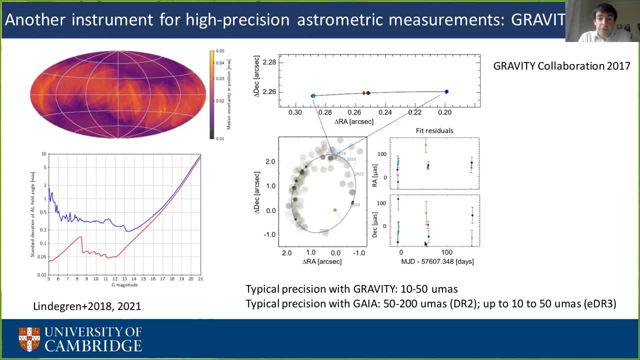 of planets, And probably the first thing which is interesting to say is that if you look at the numbers- so I have here two figures which I took from the Gaia DR3 astrometry paper and the Gaia DR2 astrometry paper- 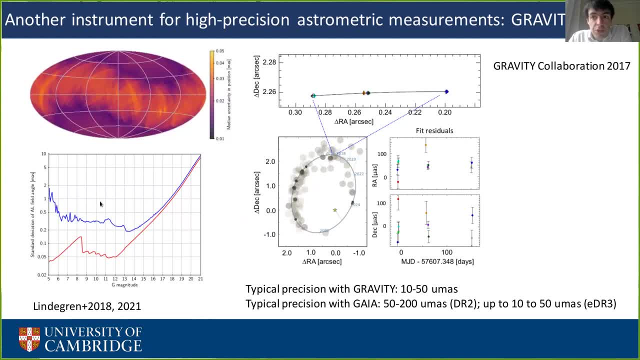 If you look at the numbers, the typical astrometric precision that you have with Gaia depends on the data release and it depends on the target, especially the magnitude et cetera, But it's typically going to be 50 to 200 micro arc. second, 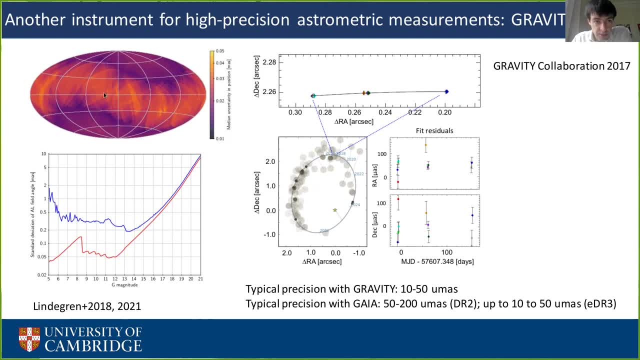 in DR2 and 10 to 5 micro arc. second, if you look at DR3, EDR3.. If you look at gravity observations, you also get a typical precision on the astrometry which is 10 to 50 micro arc. second, 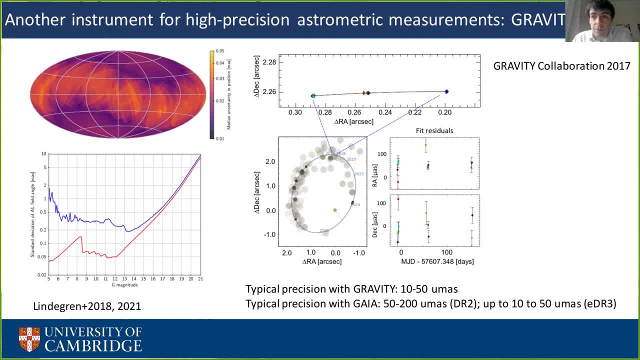 So it depends on the orientation of the baseline, depends on a number of things, but that's the broad part. Now, the difference, of course, is that, to get this level of precision, Gaia is averaging a number of measurements, whereas with gravity. 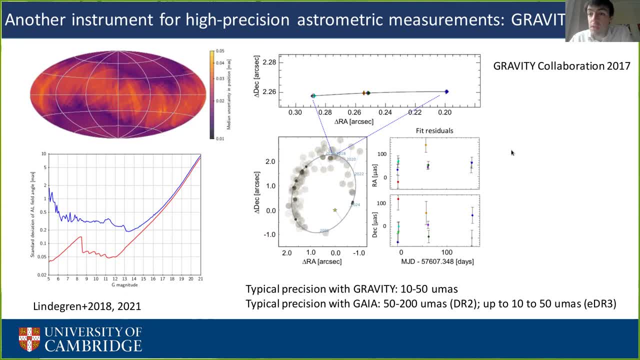 you can get this level of precision with a single epoch observation, So you observe during one night and you can get this level of precision. Now, of course, the problem is: Gaia is observing the entire sky, which is quite nice, whereas with gravity 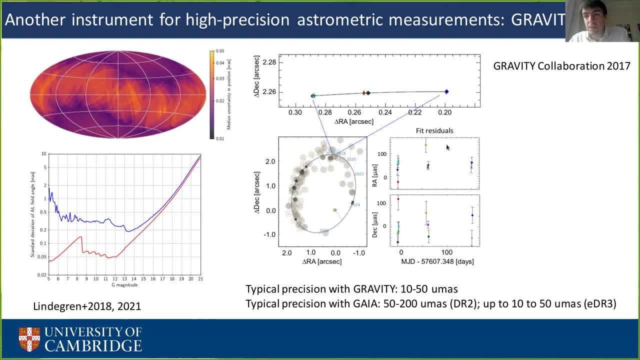 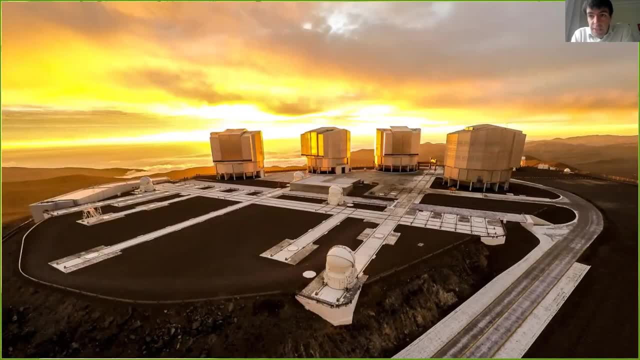 you have to observe each star individually, so it's more time consuming. But so let me talk a little bit about this instrument- gravity- because with this level of astrometric precision, there are a number of things which I think are quite interesting. 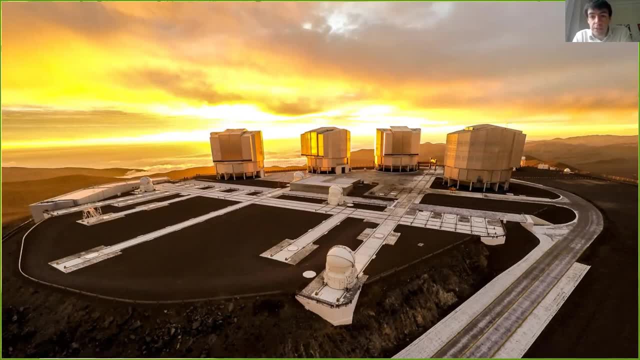 to do for exoplanet detection. But I need to talk a little bit about the instrument in order to be able to talk about the advantages and the problems it raises. So gravity is an instrument on the very large telescope interferometer so it can combine the lights. 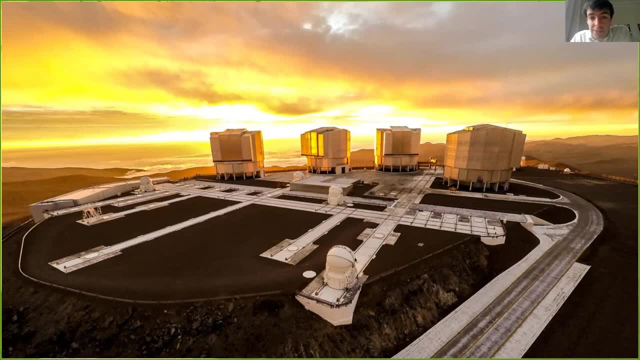 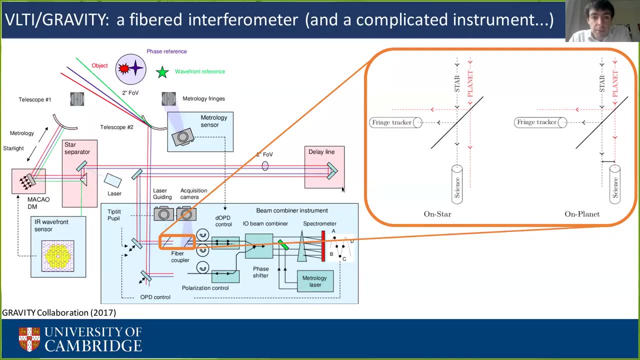 coming from the four-unit telescopes or the four auxiliary telescopes, And so it's quite a complicated instrument. so I'm not going to go too much in the details, but I need to talk about a number of things. So it's a fibered instrument. 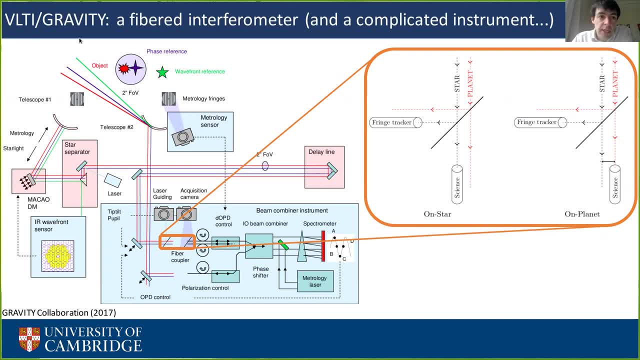 it's a fibered interferometer. So the way it works is: the light comes to the telescope, it's collected by the telescope, then it goes to the delay lines of the very large telescope interferometer, then it goes to the instrument- gravity- itself. 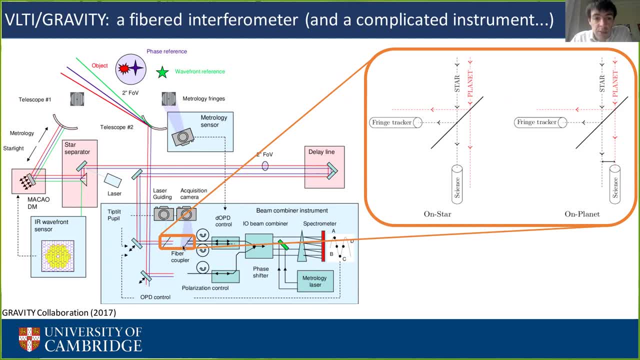 and here you have a. the light is injected in single-boot fiber. then you have an OPT control system where you can control the optical path difference between the different telescopes of the array. and then it goes to the beam combiner and to the spectrometer. 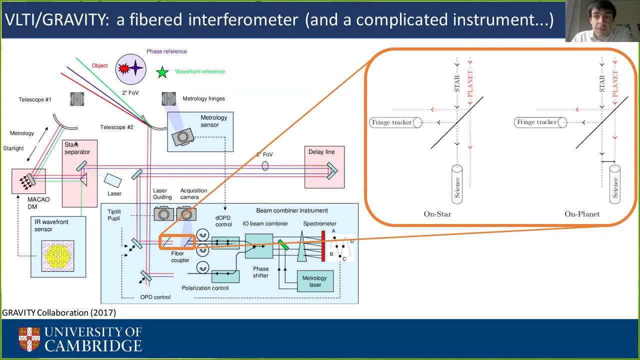 Now in the instrument. so there is also adaptive optics on the telescope. so part of the light goes to the adaptive optics system. So it's an AO-corrected fibered interferometer. Now there are in the instrument two channels. One is the science channel. 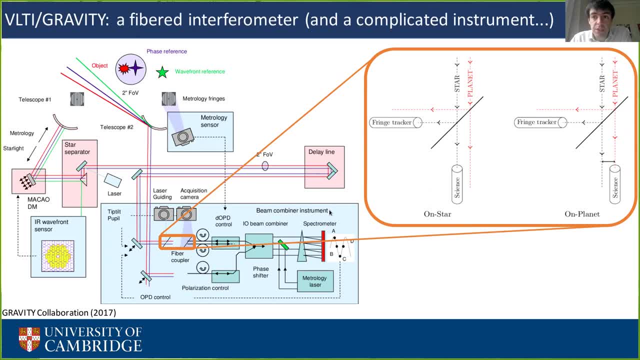 on which you get your science measurements, and the other one is the fringe tracking channel, And the idea is the fringe tracking channel is used to correct the phase errors coming from the atmosphere. So basically, the role of the fringe tracker is to sort of freeze. 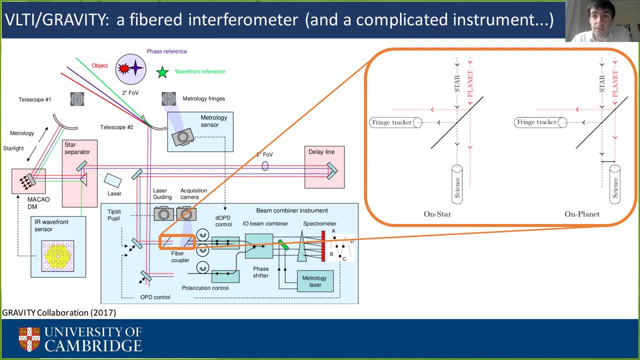 the atmospheric turbulence in terms of phase, so that you can do long integration on the science channel and the fringe tracking channel. So this is extremely important because then you can get rid of this atmospheric distortion of the phase. The problem is between the science channel. 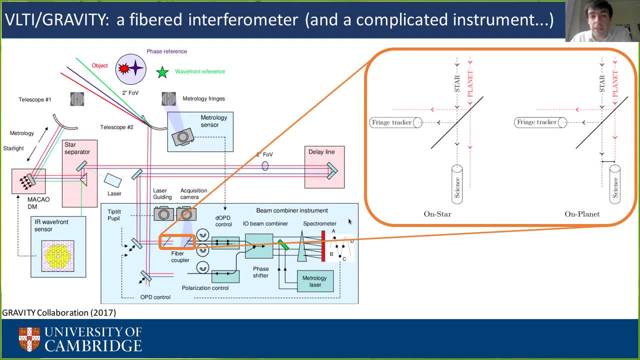 and the fringe tracking channel, you can have non-common path errors. So you don't have a good measurement of the phase of your object with this, which is why in gravity there is also a metrology system. So there is a laser which back propagates. 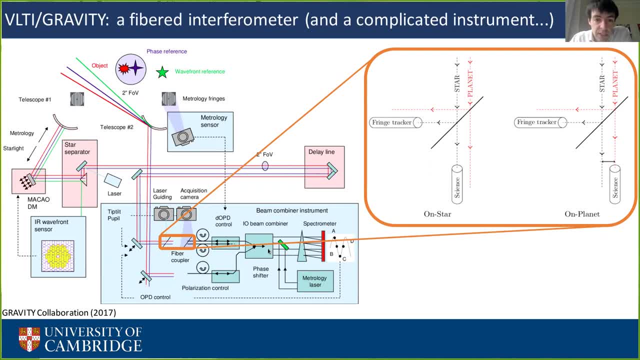 into the entire optical train, So it's injected in the science and fringe tracking fiber for each telescope. It back propagates into the entire system all the way to the telescopes, And at each telescope there is a set of diodes on the spider of the telescope. 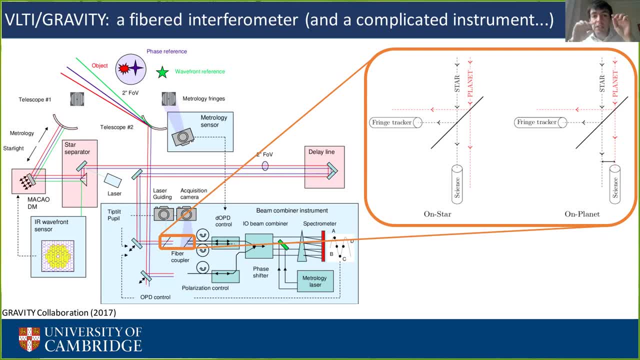 which basically those diodes are going to see an interference pattern from the light of the laser coming from the fringe tracking fiber and the science fiber And with this you can actually measure the non-common path errors in the system. And if you combine all of this 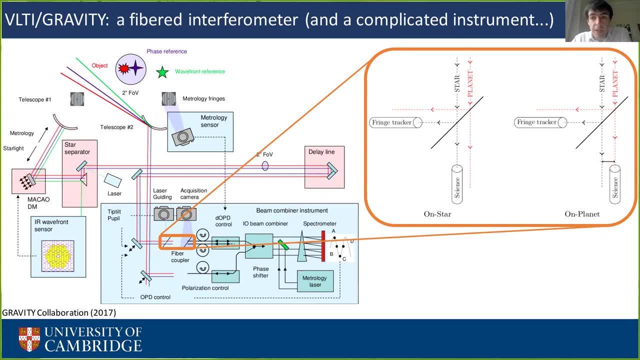 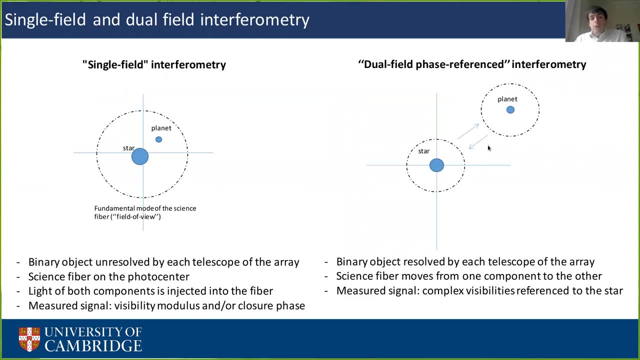 you can actually get measurements of the phase of the object that you're observing to. there's just an unknown reference point, basically, which is important. I'm going to come back on this later on. So there are different ways to observe with this instrument. 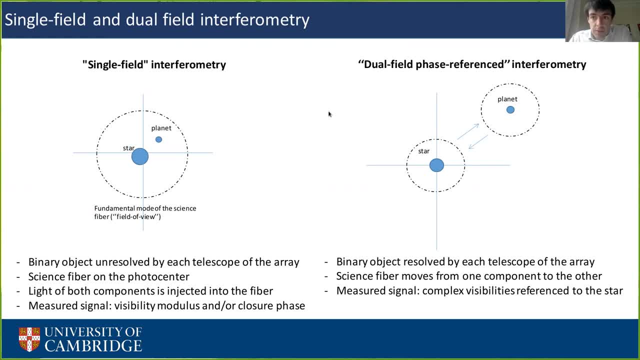 One of them- and this is very relevant to what I want to discuss- which is detecting planets with trauma. So one of them is observing in single field mode, So where, basically, you're trying to look at a binary. I took this example. 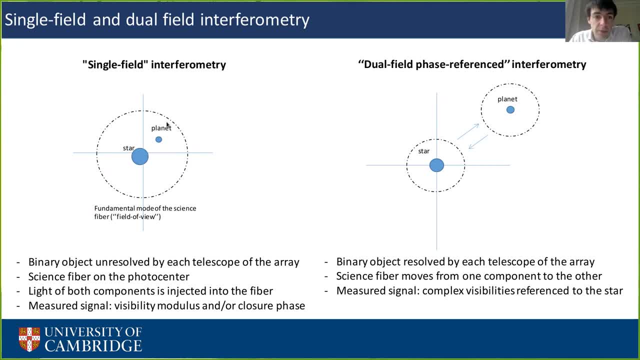 a star in the planet, It could be a double star, It could be some other objects, But you're trying to look at something which is below the resolution of a single telescope of the object, Which means that the light of the entire object or the entire system, 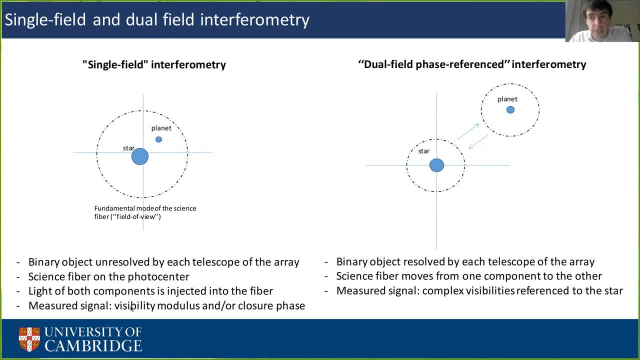 that you're observing goes into the fiber, And then you get information on the spatial distribution of the flux from the interferometric measurements. The other way you can use the instrument is in a mode which we call dual field phase-referenced interferometry. 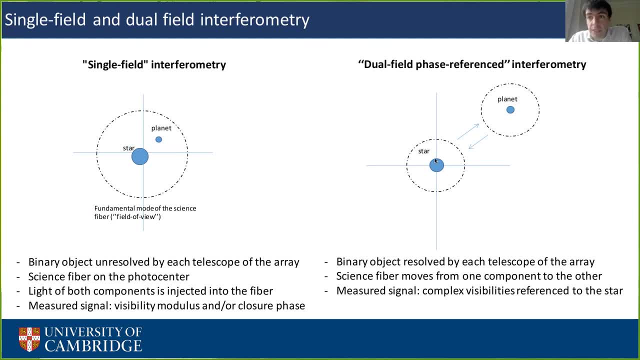 where, basically, you're observing a system which is above the diffraction limit of a single telescope. So you put your science fiber on, for example, in this case the star, and then you move the fiber to the planet and back to the star. 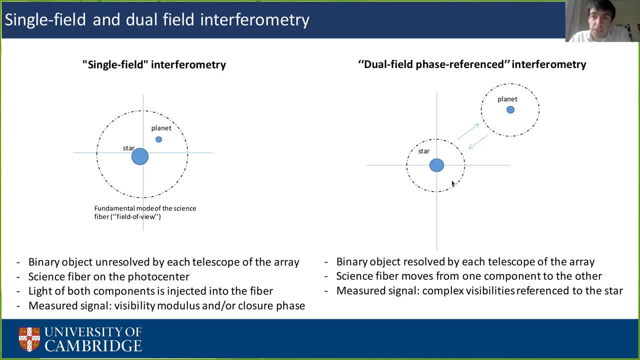 to the planet, etc. And in this mode. so this is something that you can use only because there is this entire metrology laser system, and all of this Because, in principle, if you have only one object in the fiber, you cannot measure. 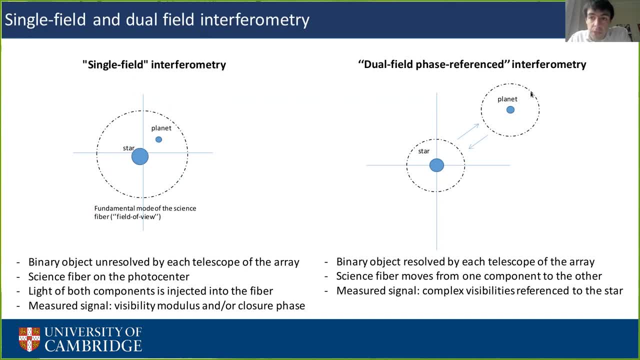 the relative astrometry between the two. You can only do this because you have this possibility of phase-referencing your observations. So if you observe like this, then in principle you can measure the relative astrometry of the two objects. 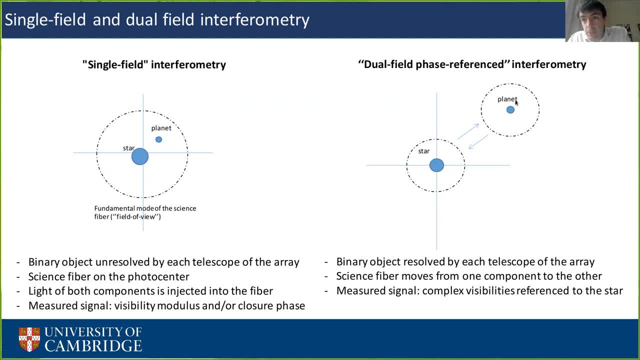 It's also very useful for the direct detection of exoplanets, because, of course, if you observe in single field mode, then basically you have all the light from the star injected into the fiber, Whereas if you observe like this, when you put the star 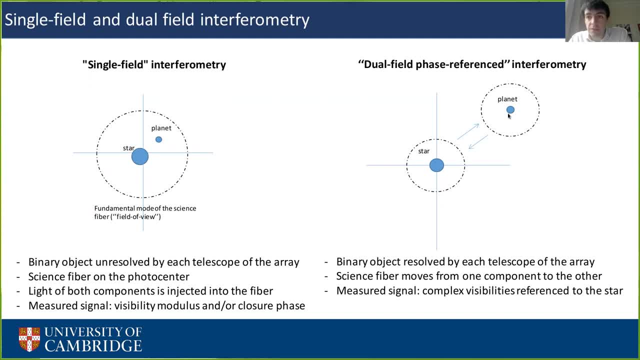 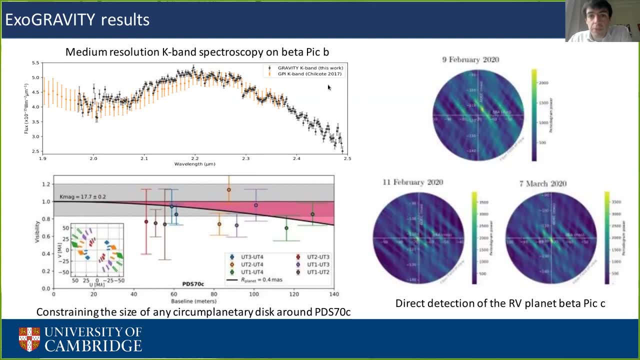 the fiber on the planet, then you filter out a significant fraction of the stellar flux. So this is the mode that we've used in the ExoGravity LARGE program, with which we got a number of results so far. So, for example, medium resolution. 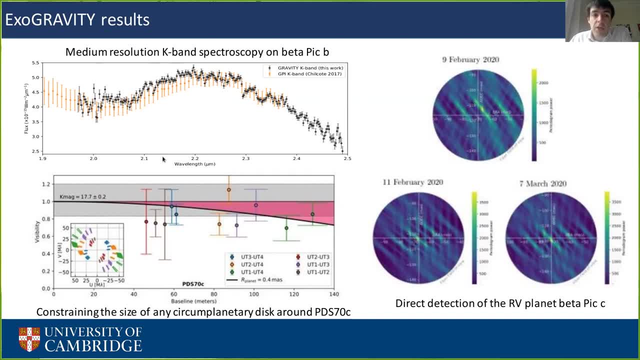 K-Band spectroscopy on bit of bit b observations of PDS 70 b and c- actually I just put a plot here from a paper by Jason Wong- And of course the direct detection of the radial velocity planet bit of bit c. 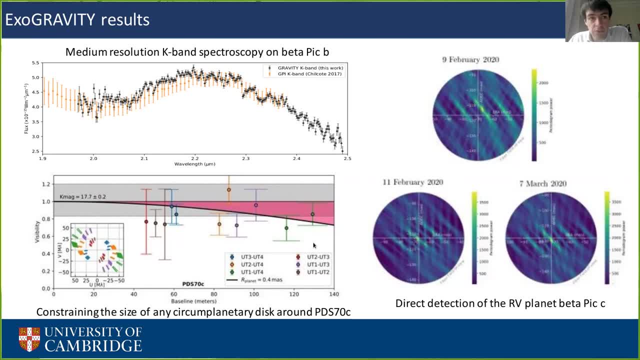 So all of those results which I'm not going to really discuss because they aren't really relevant to what I want to talk about, which is astrometry, all of those results were obtained in this mode where we move the fiber from the star. 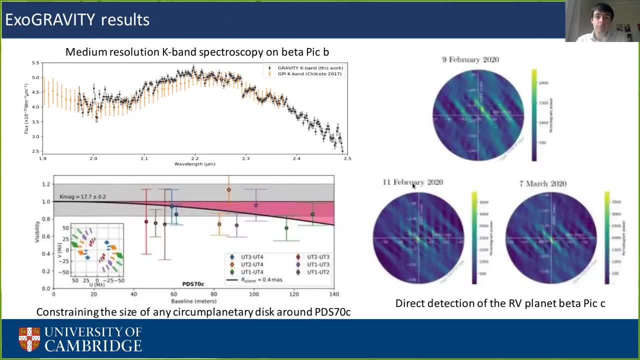 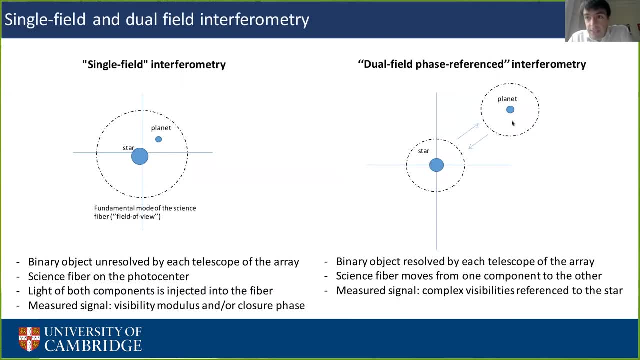 to the planet and back again on the star itself. Now, the problem with this is actually when you observe like this. So, first off, if you observe something in this mode, then basically you need the system to be below the diffraction limit. 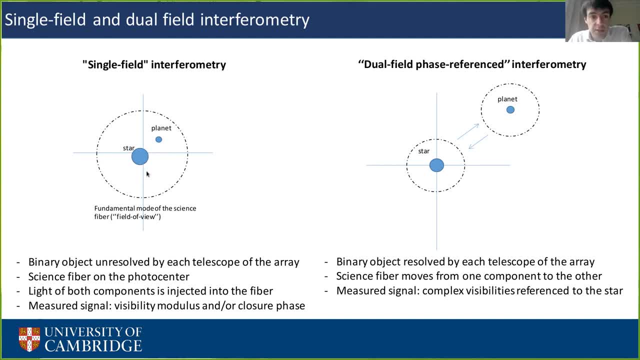 So the separation can be at most 60 ms for the unit telescope of the VMT. If you observe, in this mode, there are a number of factors in the instrument which set a hard limit on the distance between the two objects that we can observe. 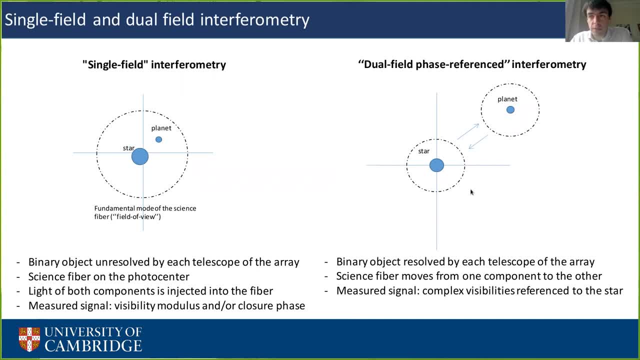 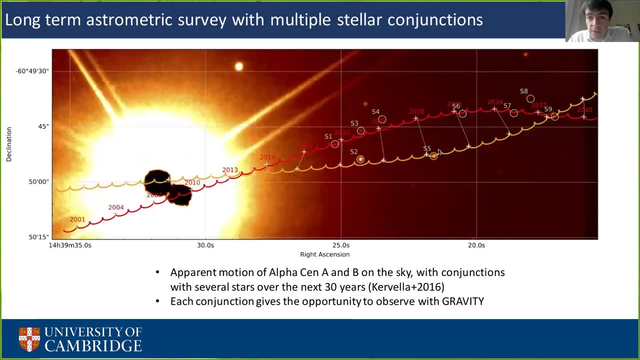 which is for gravity. it's two arc seconds, I believe. So you cannot observe, say a star here and use a reference point which is more than two arc seconds away, which means that if you want to get astrometric measurements with gravity, 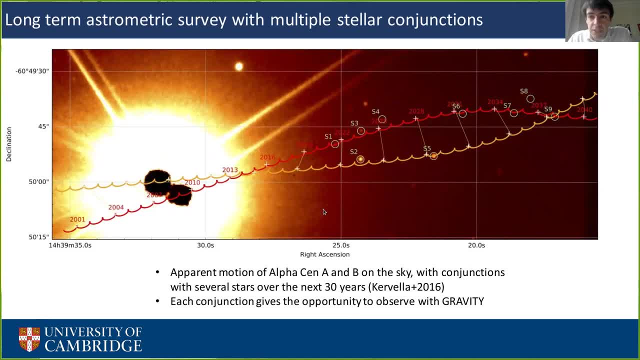 using this mode. basically, you need to observe your target and to find a reference star, which is not so. it needs to be bright enough so you can observe it with the instrument and it needs to be, at most, two arc seconds away from the target. 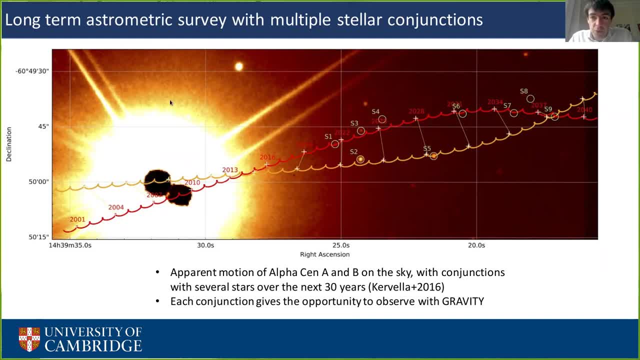 which leads to many complications, of course, observationally speaking- And this is a plot I took from a paper by Kavala in 2016.. This is the trajectory of alpha-sen A and B on the sky And on the background. 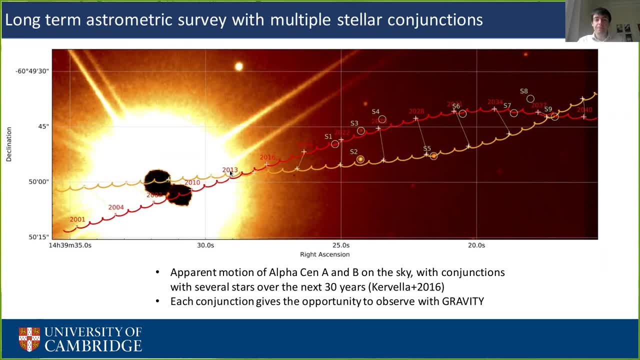 you have a J band image And you see that this is the trajectory of the star on the sky And you see, here, circled in green, you have a number of background sources which are actually the sources which can be used to do phase-referenced. 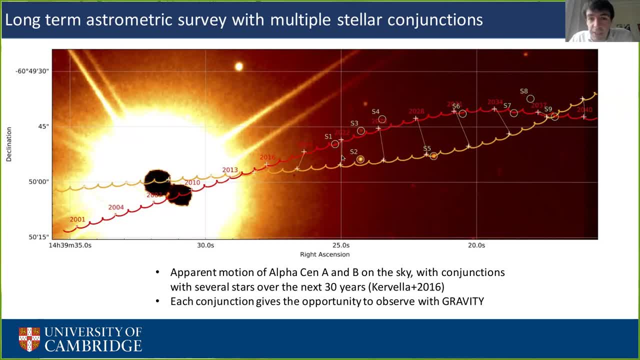 astrometry of alpha-sen A or B for the next what? 20, 30 years? 20 years for the next 20 years? So you see, there aren't that many targets which can be used And, of course, 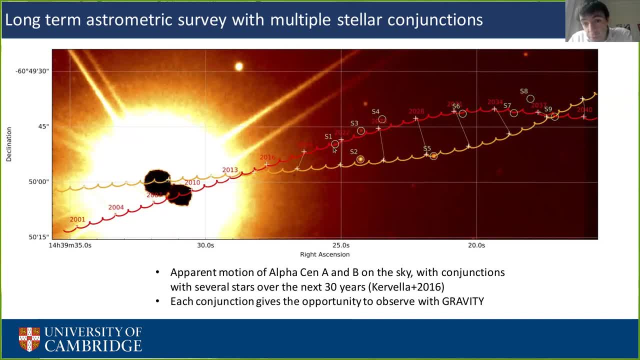 you. basically what happens here is you have a number of observing windows at which you can, which you can use to get astrometric measurements on alpha-sen A and B, But it's quite limited again, because those sources cannot be more than. 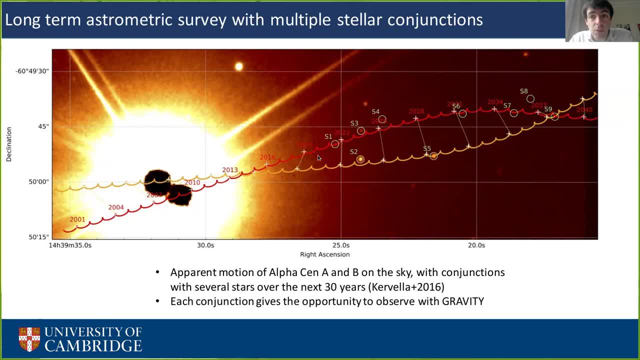 two arcseconds away from your main target. So it makes everything quite complicated to be able to do those measurements. But in principle that's feasible So you could follow those stars on those on those on those windows and get astrometric measurements. 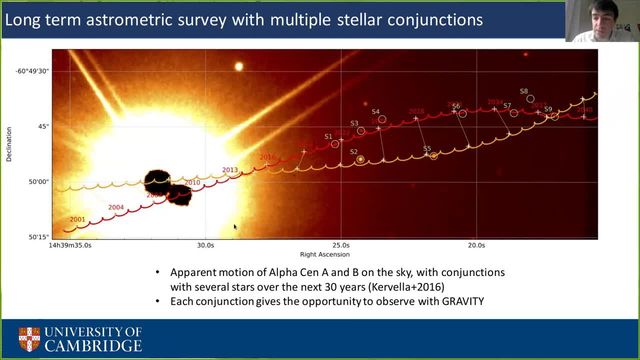 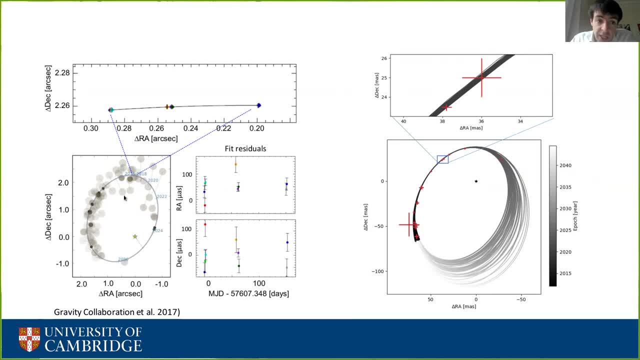 and potentially detect planets around those stars. The other thing you can do is you can observe a binary. If you have a binary star, then you have an obvious, so you can observe. you can measure the relative astrometry between the two components. 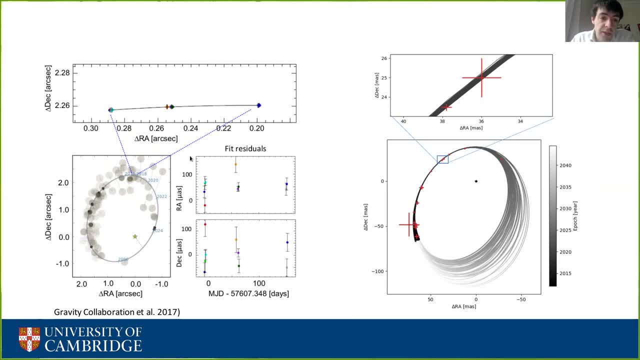 of the binary And you can measure the orbit of the binary. So those are two examples Now, two binaries on which we can measure the orbit. Again, you have the measurements at the precision of gravity, so typically 50 micro arcseconds. 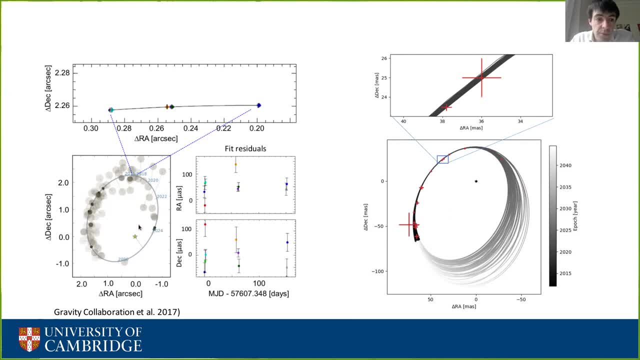 And you can try to see a deviation from the two-body Keplerian motion generated by a planet orbiting around one of the components of the system. Again, you need a binary which you can observe. So the two components need to be at most half a second. 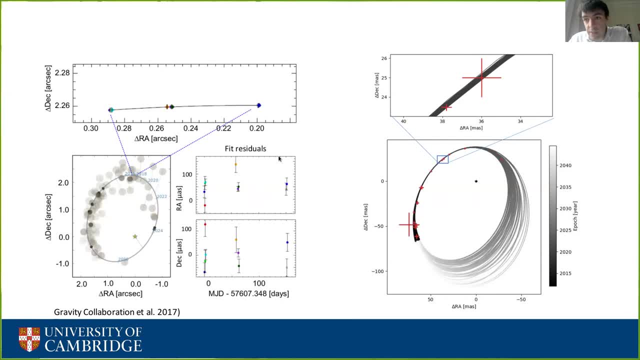 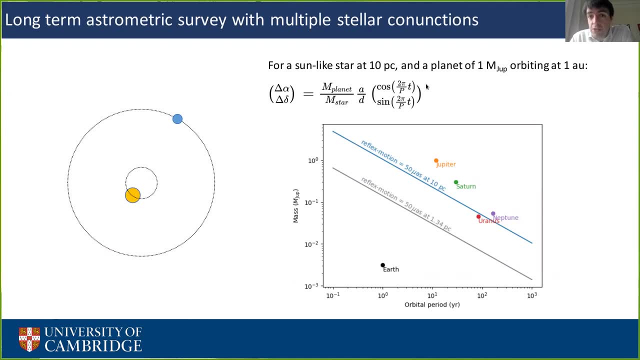 away from each other. Next, it's complicated, but in theory that's feasible. Now the interesting part is with gravity. you have a measurement at this level of precision: 10, 50 micro arcseconds at each epoch at which you observe. 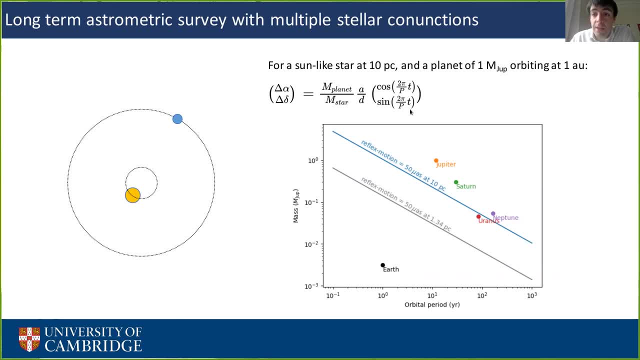 So if you look at the numbers, in theory this could be a very powerful method. If you look at a star which is a sun-like star at 10 or 1.34 parsecs, you can see that the number of stars. 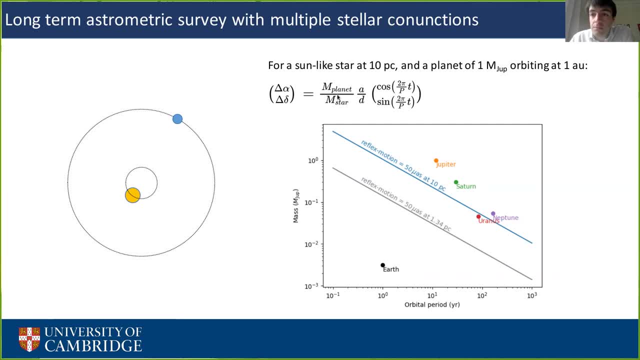 is very small And you look at the typical mass, planetary masses that you can hope to be able to detect with this level of precision. then you get to masses which are, which can be a fraction of a nuclear mass. So that can be. 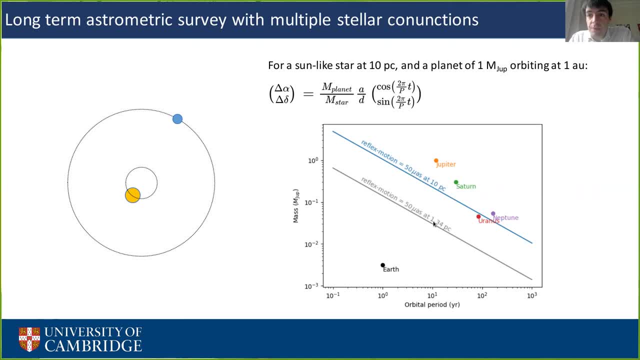 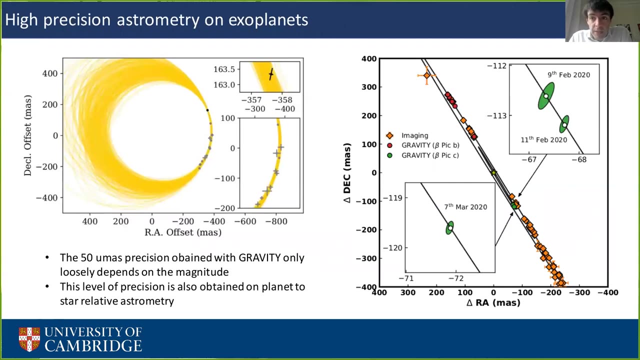 a very powerful method. It wasn't for the difficulty of doing the observations, because you need this reference point, this reference target, this reference point. Now, interestingly, even when we observe exoplanets, which are relatively faint targets, we do have. 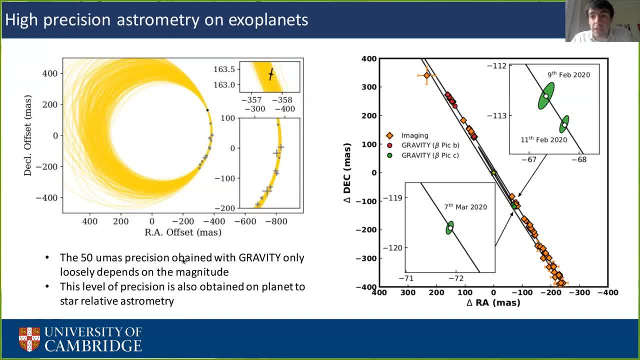 the same level of precision on the astrometry. We do have astrometry at a level of 50 micro-arcseconds on those observations of exoplanets. We've demonstrated this on HY8799E and also on BNC And you can. 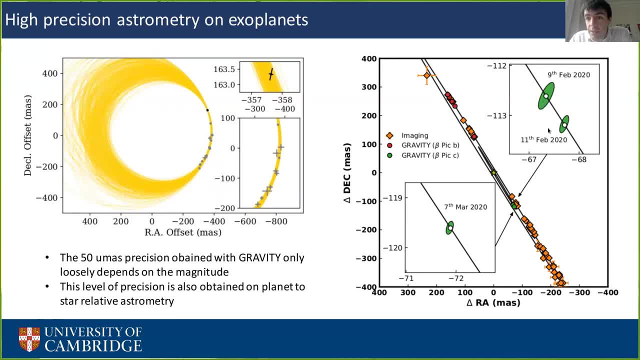 see the gravity astrometry of Betapix C on the 9th, 11th and February 2020 and on the 7th of March 2020.. And it's quite amazing actually, We can already see the motion of the. 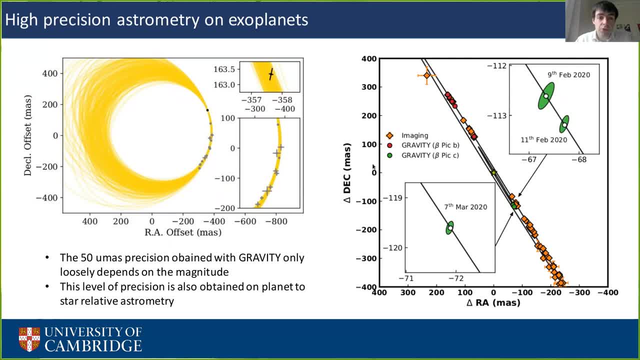 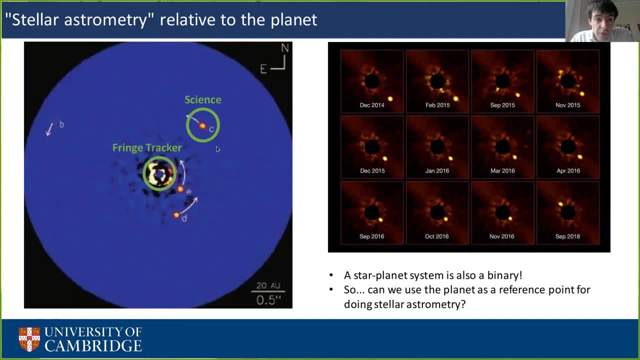 planet, even between those two epochs, on the star. So if you think about it, if you have the star and a planet orbiting around the star, you can observe the system. So put the fiber on the star or put the science fiber on. 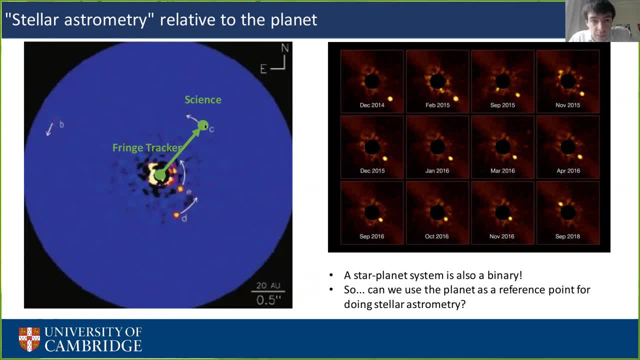 the planet and then you move back and forth And then you would measure the relative motion of the star And you can see that the star is moving a little bit because of the reflex motion caused by planet C. So the star is orbiting on an 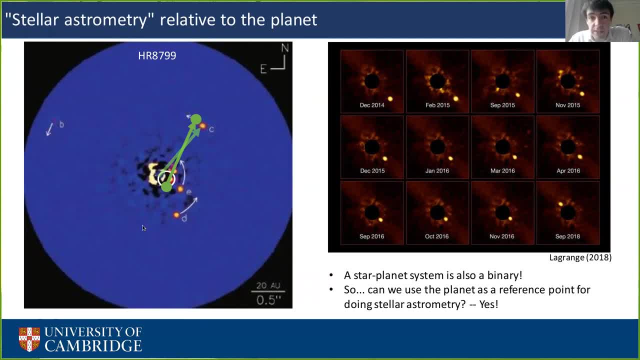 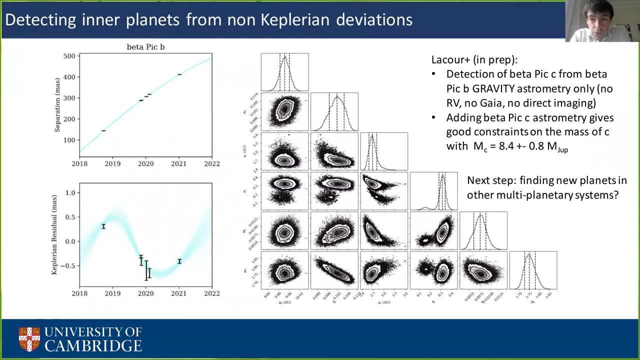 orbit generated by this planet E. So, in principle, this relative motion of the star plus the planet around it is also a binary system which is easy to use because usually the planet is at less than two odd seconds away from the star. So this 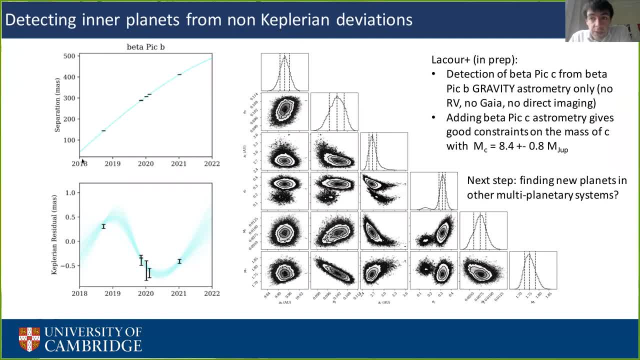 is something which we are currently doing with gravity, especially on the Betapik system of Betapik B. so two-body capillary motion And you subtract this, then you can actually see in the residuals the reflex motion of the star generated by C. 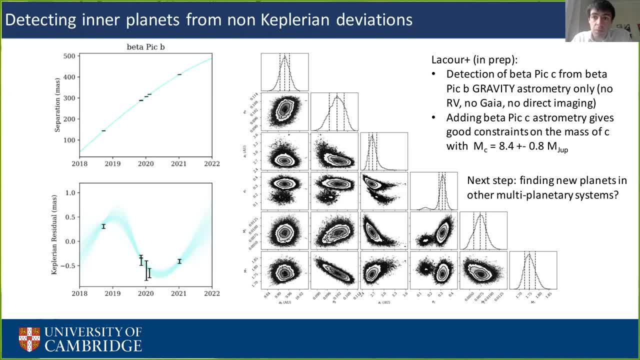 which means that we are at a level with gravity where we can detect planet C only using astrometry on planet B. so you can- in principle you could- measure the mass of C doing this. Now the error bars are quite big, but in 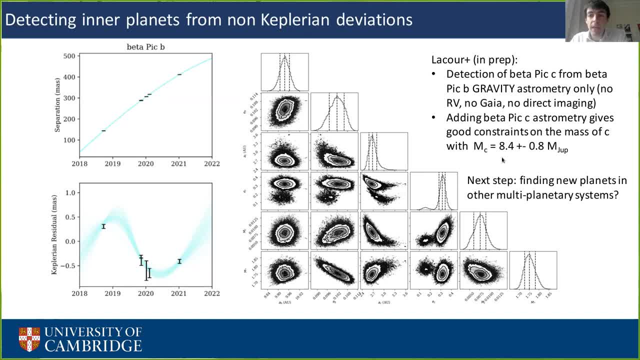 this case because we also have an astrometry on Betapik C. if you add this into the mix, then you get a good measurement of the mass of C. So basically, what we are trying to do is to do this. 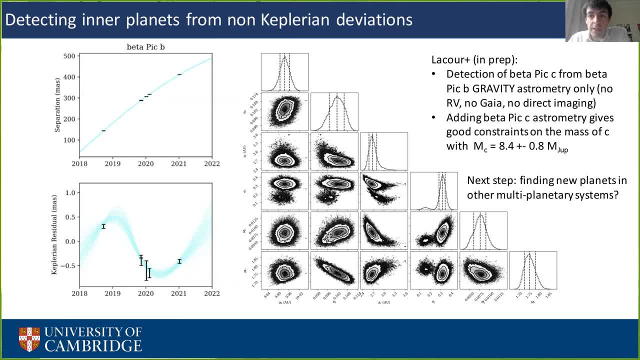 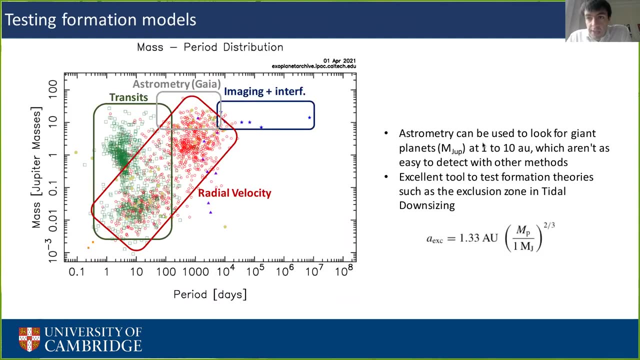 on other systems and to try if we can detect new planets in known planetary system just by looking at the astrometry of the external planet. So basically, following this, we take a step back and talk a little bit about why this is useful. 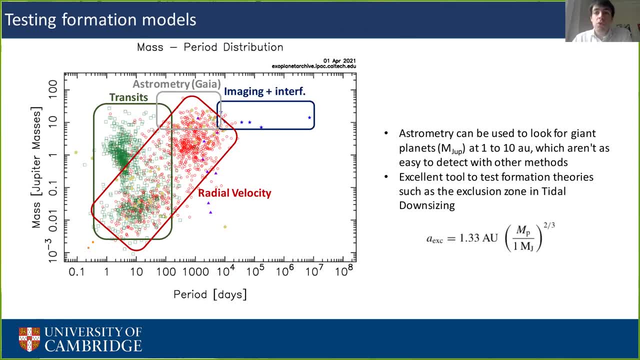 basically because there are other methods to detect planets. so why is it interesting to also look for planets using astrometry? And I think there are a number of answers to this. One of them is that the range of masses and periods at which 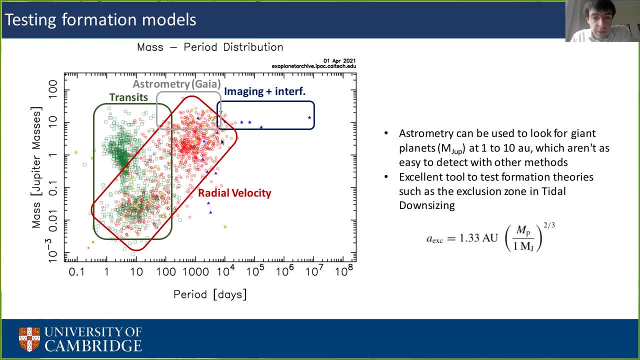 you can find planets is typically a couple of Jupiter masses and above or below for some targets and a semi-major axis of a few astronomical units. Now for some formation theories, and I'm mainly thinking about the exclusion zone, which is basically a limit. 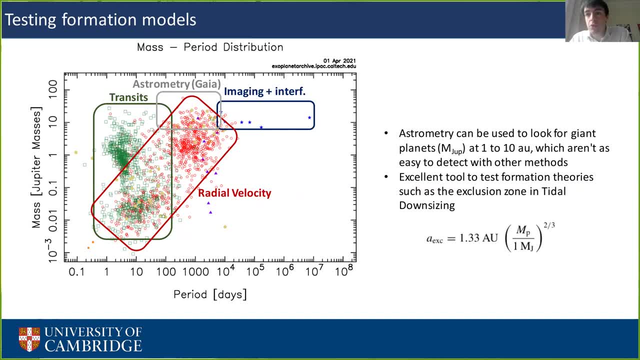 at the semi-major axis, below which you cannot find- or it's more difficult to have- giant planets. Now this: if you do the calculations for plugging the numbers, you would find that if you want to measure the mass of the planets, you would. 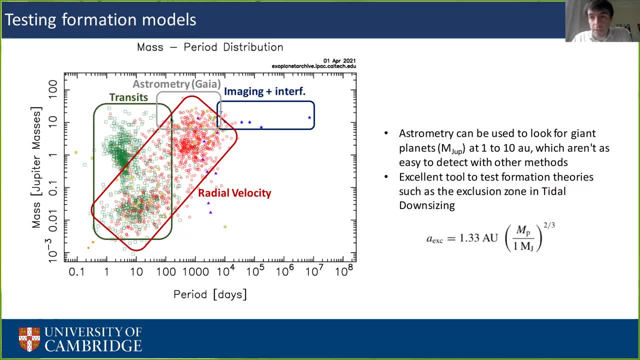 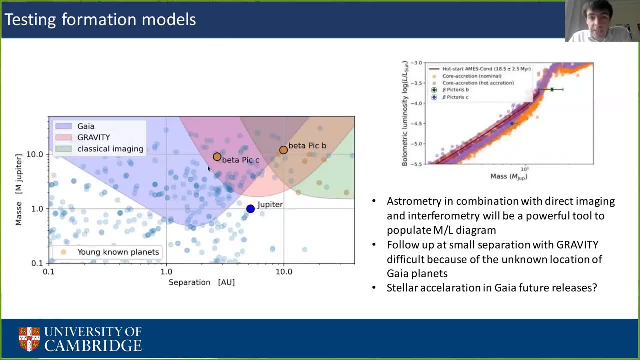 have to measure the mass of the planets, which is best probed by this combination of astrometry, with Gaia at the surface. Now, if you look also at the different Gaia observations, you can measure the luminosity of the planets. 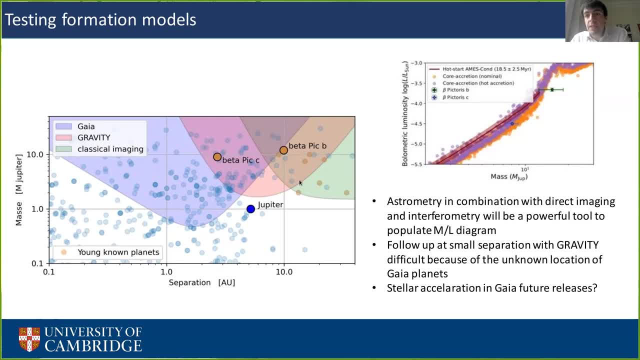 And we all know that the mass luminosity diagram can be a very powerful tool to test the planet formation theories and the cooling tracks and all of this. So this could, in principle, be followed up by direct imaging of gravity. Now again, 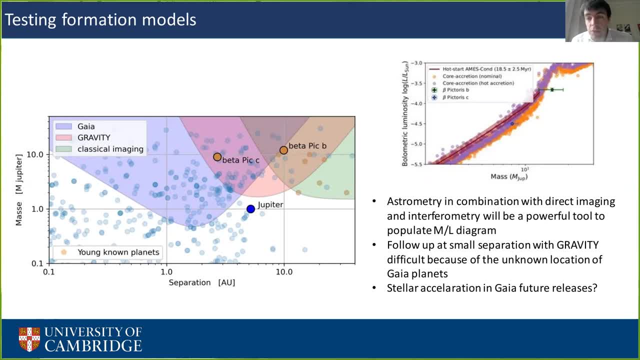 the problem with gravity is you need to know where is the planet if you want to be able to observe it. So it's a very powerful instrument because you can observe at small separations, but you need to know where it's going Now. 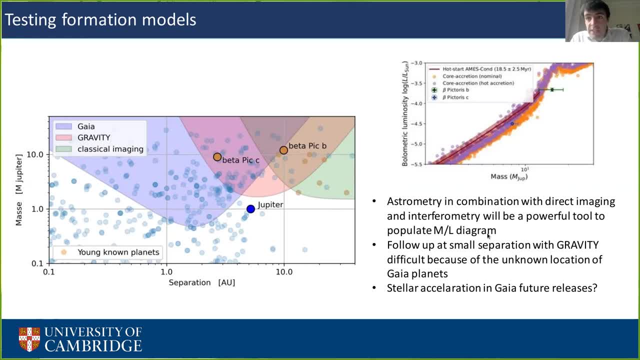 on young targets that you can observe with direct imaging or gravity. it's hard to get rid of velocity data, so then we need to find a way to be able to guess the position of the planet from stromatic measurements. So we need to know. 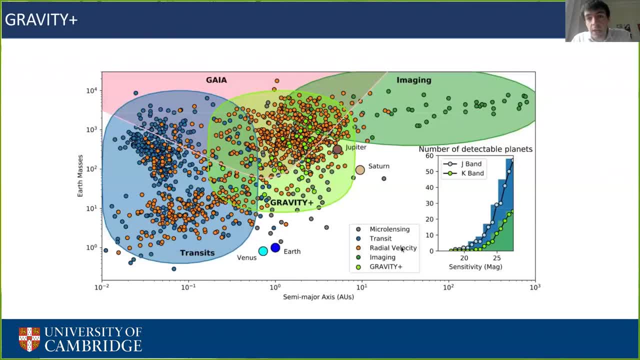 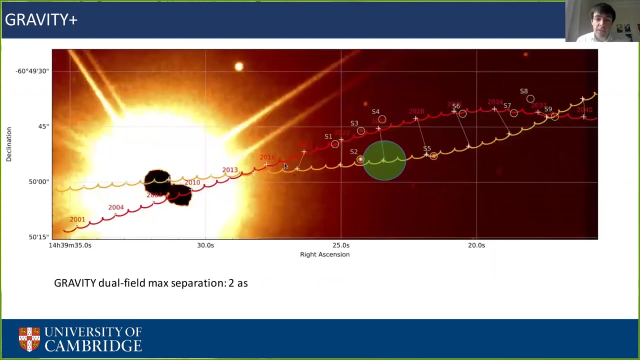 where is the planet and how to predict the location of the planet and to follow up with gravity, And so we have an updated version of gravity in the future which should improve the capabilities of the instrument, so that should really help to extend the